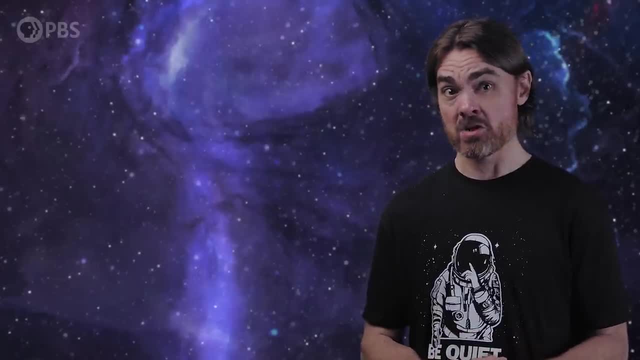 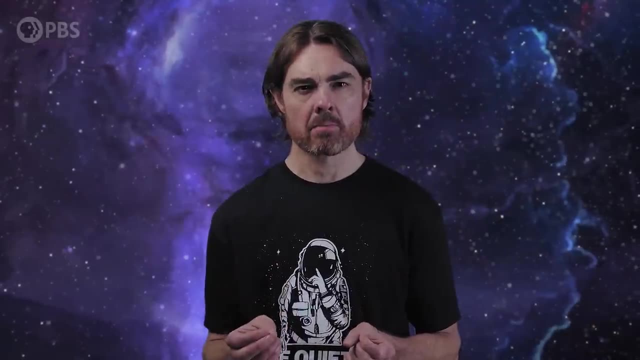 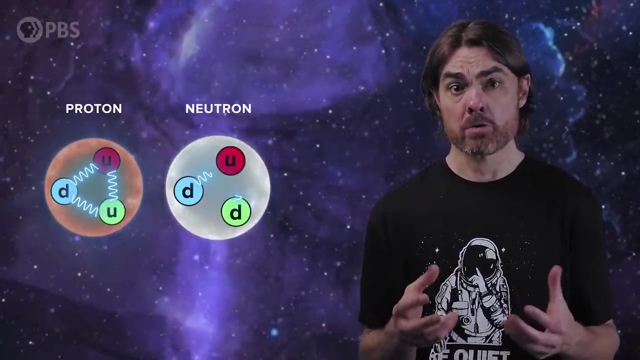 molecule. We also talked about the hack that lets us do that anyway. It's called density functional theory. DFT is good for simulating the electrons in an atom, but the behavior of electrons is comparatively baby stuff compared to the atomic nucleus. Every proton and neutron is composed of. 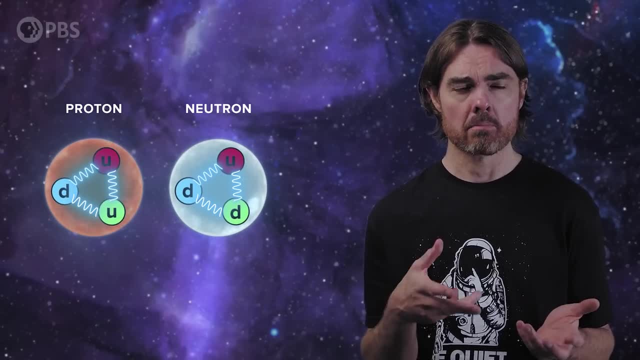 three quarks stuck together by globes. Every neutron and neutron is composed of three quarks stuck together by globes. Every proton and neutron is composed of three quarks stuck together by gluons. Well, actually that's a simplification. Every nucleon is a roiling, shifting swarm of 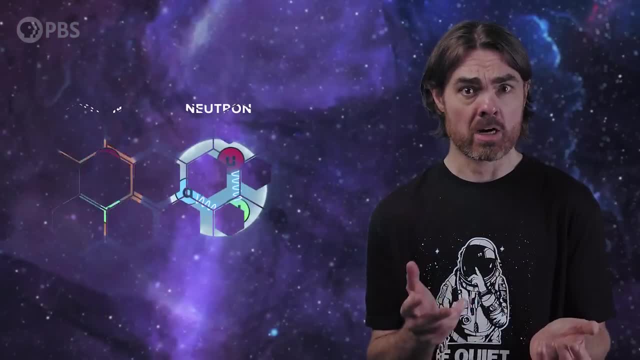 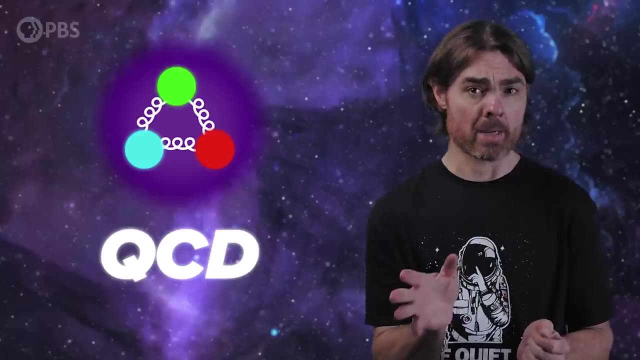 virtual quarks and gluons that just looks like three quarks from the outside. The messy interactions of quarks via gluons is described by quantum chromodynamics or QCD, in the same way that quantum electrodynamics describes the interactions of electrons and any other. 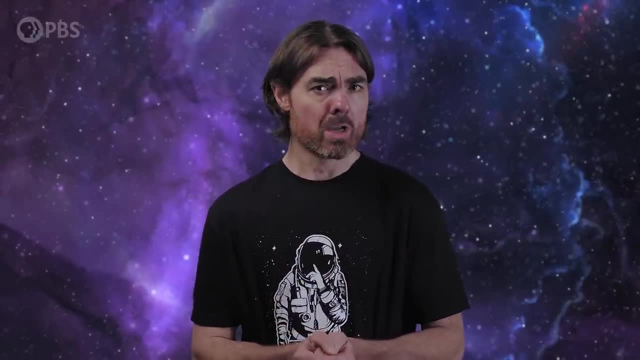 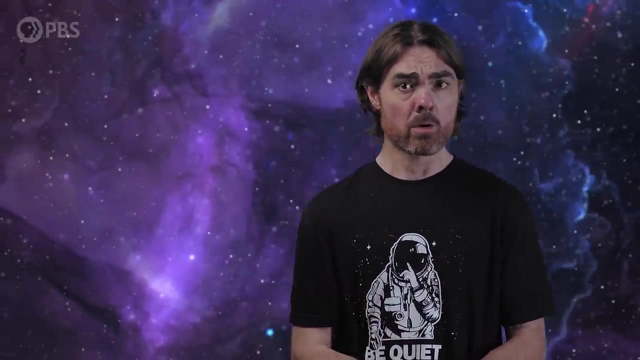 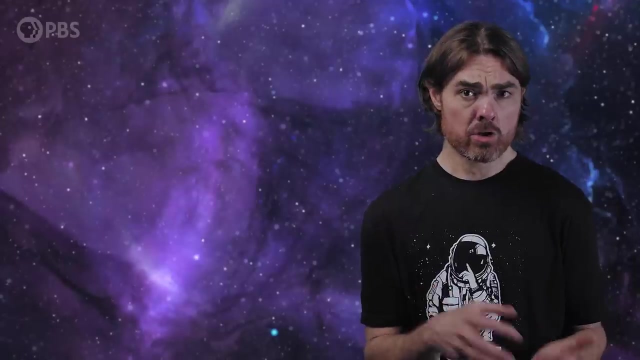 charged particles via photons. We're going to come back to a full description of QCD very soon, but you don't need it for this video Today. we just need to understand why it's complicated. Instead of the one type of charge in QED, in QCD there are three, which we call. 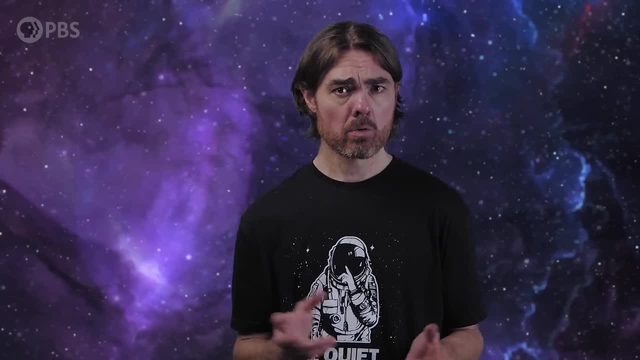 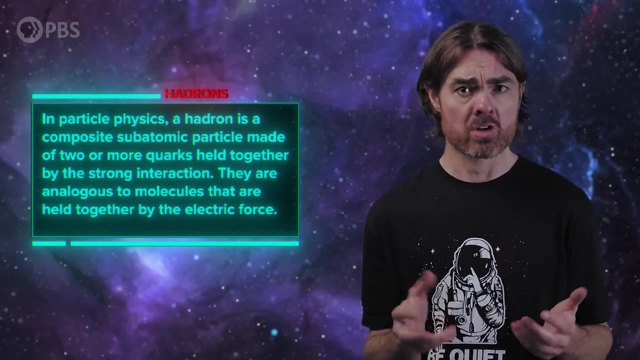 color charges, hence the chromo in chromodynamics. Also, quarks never appear on their own. they're always bound to other quarks in composite particles called hadrons, of which protons and neutrons are an example. To test QED, we can chuck a photon. at an electron and see what happens. But to test QCD we can't just poke a quark with a gluon. instead we need to figure out what the theory predicts about the properties of hadrons that are actually measurable. And that's near impossible because of a third problem. 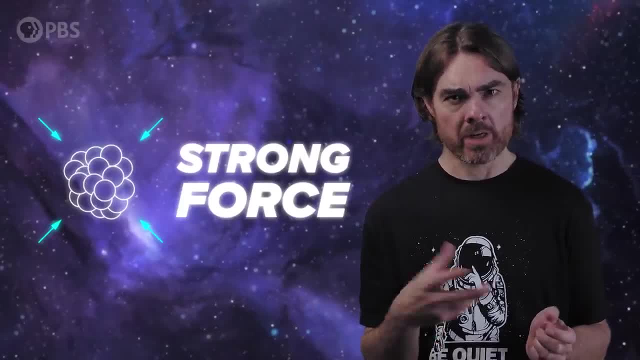 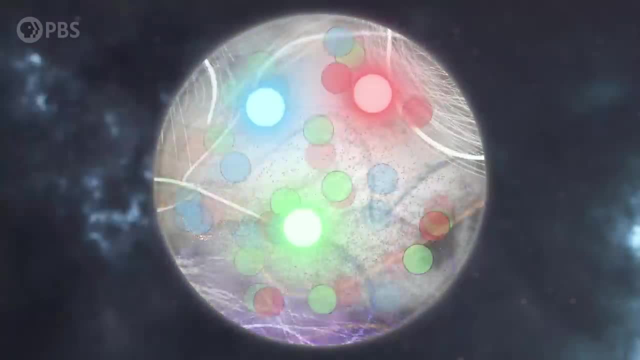 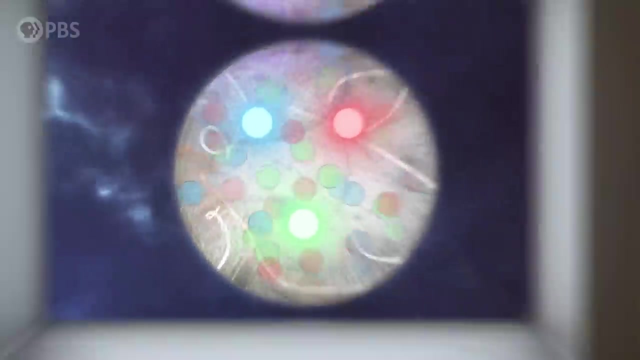 The force mediated by gluons is very strong, earning it the name the strong force. And that strength turns the interior of the hadron into a maelstrom of activity which can't possibly be calculated on a blackboard and at first glance looks impossible to simulate on any computer. 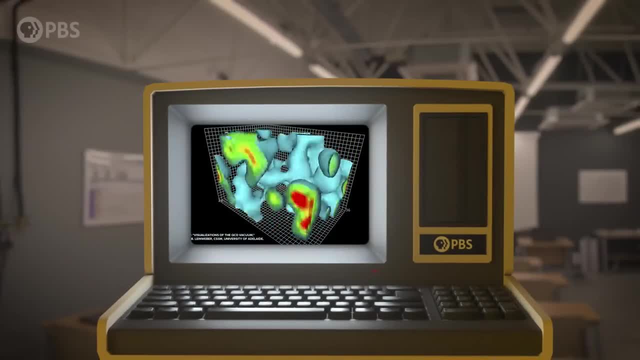 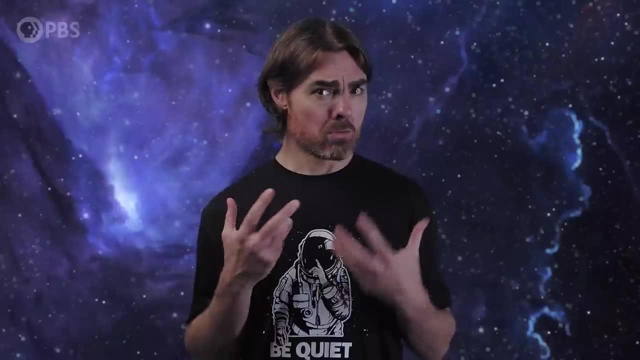 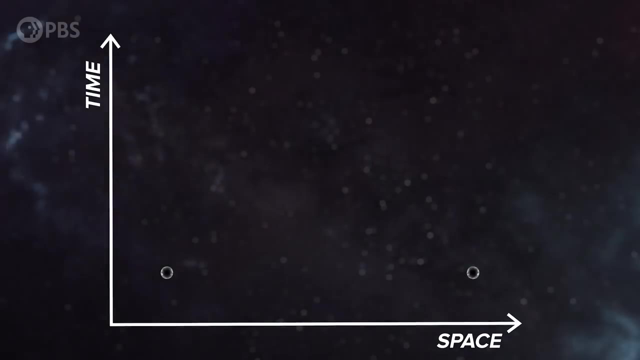 we could ever build Or would be, if it weren't for the fact that people are exceptionally clever and they came up with lattice simulations. Now, before we do the hard stuff, let's review the comparatively easy. quantum electrodynamics Say we want to predict what happens when two electrons. 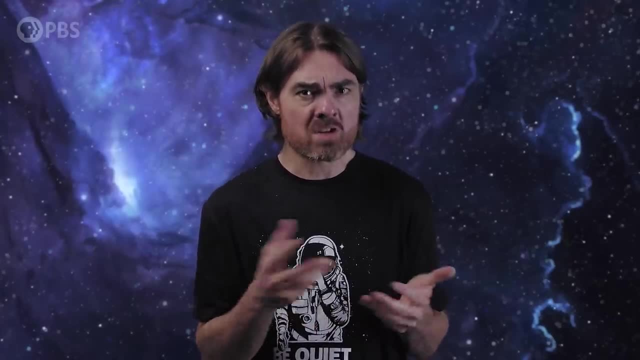 are shot towards each other, We can actually calculate the almost exact probability of them bouncing apart. and then we can calculate the force mediated by the force mediated by the electron at a given speed and angle. We do that by adding up all the possible ways that interaction. 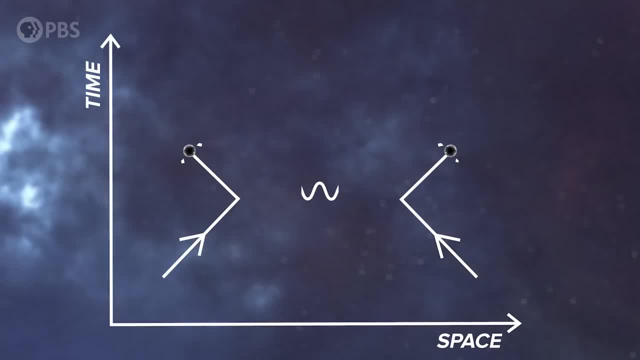 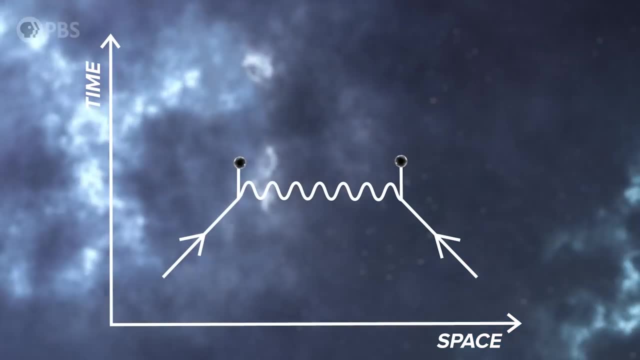 could happen. For example, there are various ways that the first electron could emit a virtual photon which is absorbed by the second electron, or vice versa. Or it could happen via two virtual photons or more, Or one of those photons could spontaneously form a virtual electron positron pair. 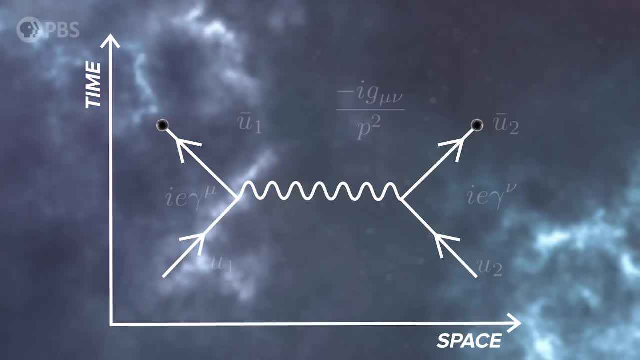 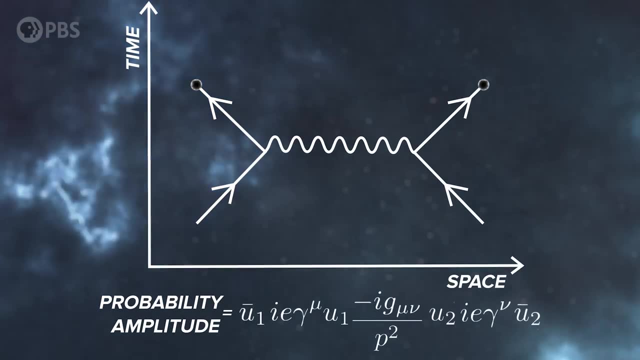 before becoming a photon again, and so on. Each family of interaction types is represented by a Feynman diagram, and quantum electrodynamics can be used to predict the force mediated by the force, mediated by the force mediated by the force. We talked about this stuff in some previous videos. 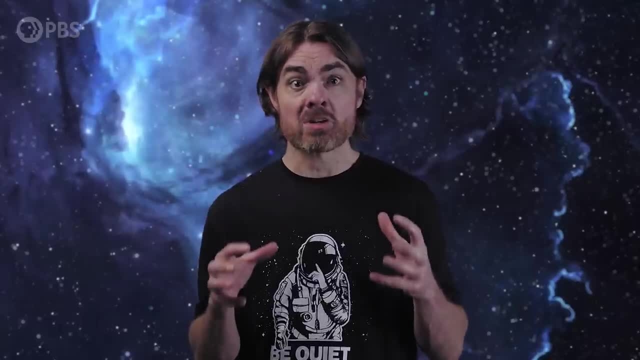 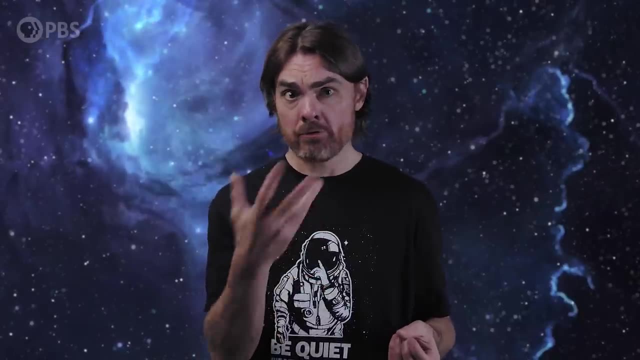 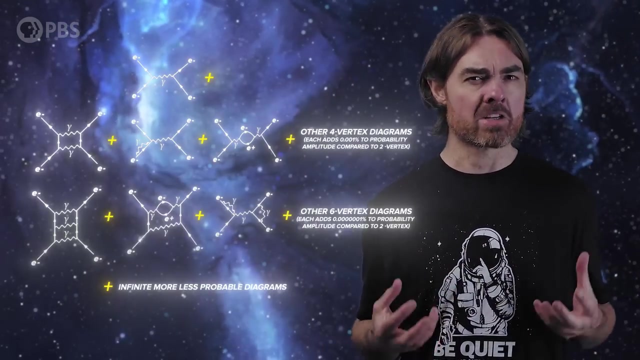 but there are literally infinite ways this interaction could happen, each more complex than the last. So how do you know when to stop adding up your Feynman diagrams? Well, we kinda got lucky with that in the case of QED, As the interactions get more complicated. 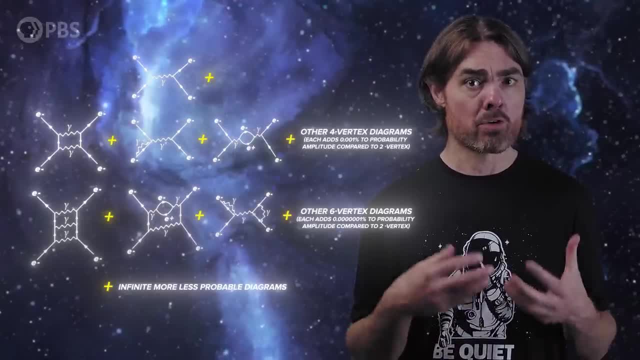 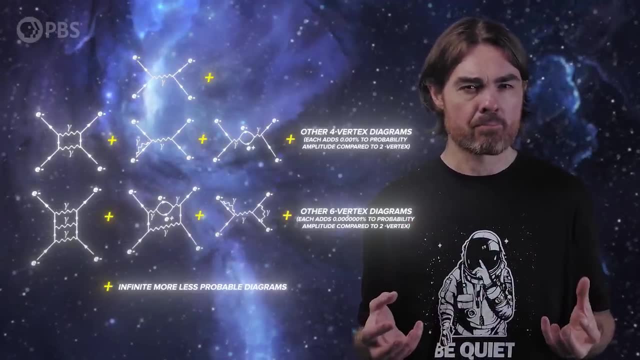 their probabilities get smaller and smaller. Diagrams with more than a few twists and turns add almost nothing to the probability, so we only have to include the simplest few levels. Each pair of vertices on a Feynman diagram represents the probability of a pair of 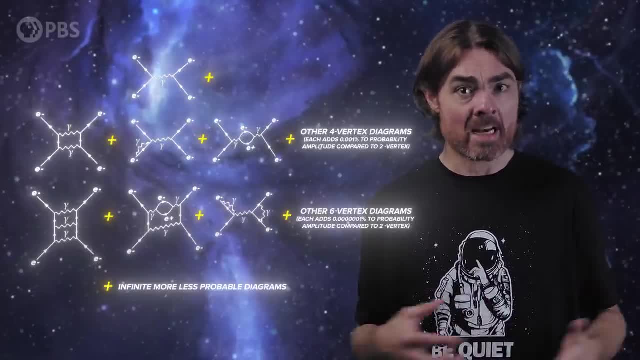 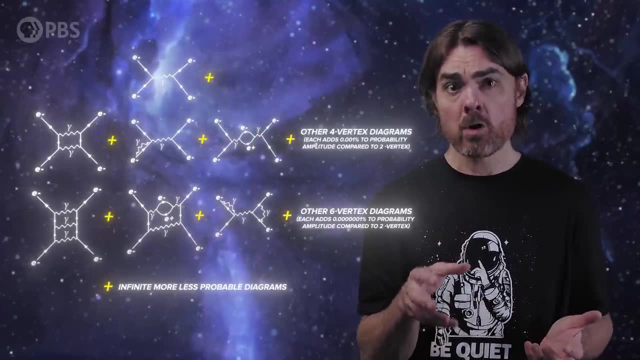 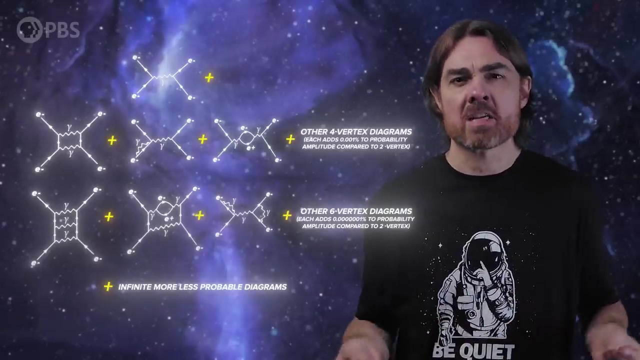 electrons interacting with the electromagnetic field, emitting and absorbing a virtual photon, And there's a set probability of that happening each time It's around 1 over 137.. So every time you add another pair of vertices to a Feynman diagram, the interaction it represents 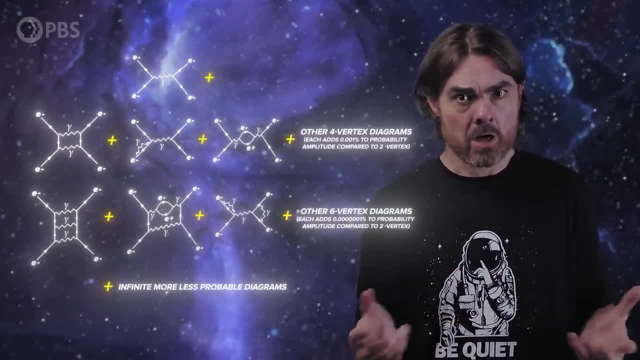 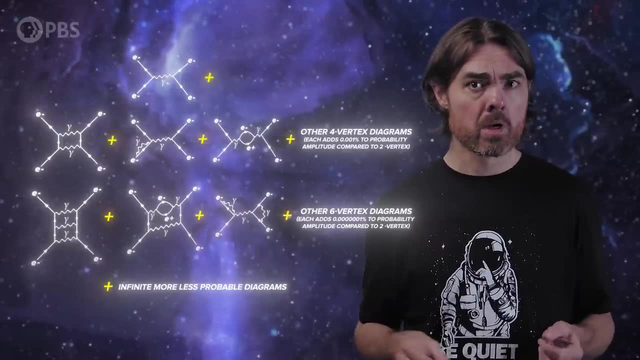 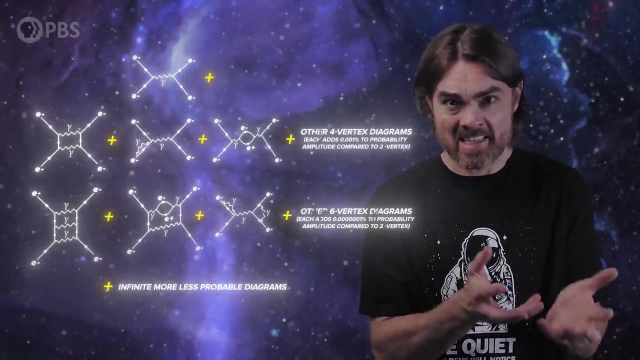 becomes 137 times less likely. A diagram with only 6 vertices is nearly 20,000 times less likely than the simplest 2-vertex diagram. So we just choose the precision we want for our calculation and ignore any interactions that nudge the probability by less than that precision. 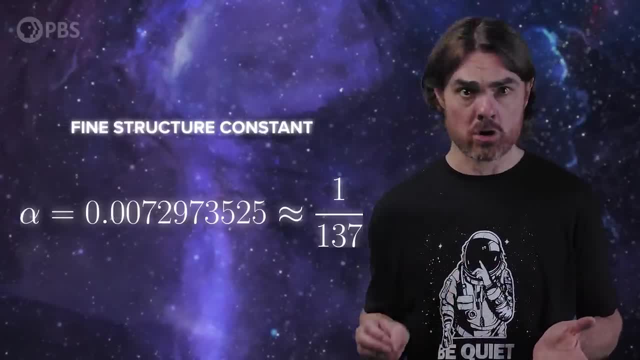 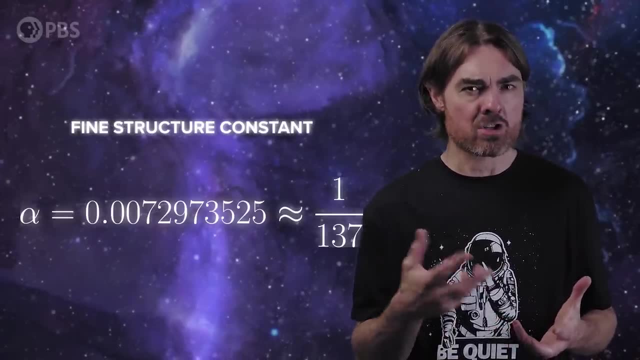 This 1 over 137 thing is the fine structure constant. It's the coupling strength between the electron and the electromagnetic field. The smallness of the fine structure constant means the electromagnetic interaction is relatively weak, Relative to the strong force anyway. 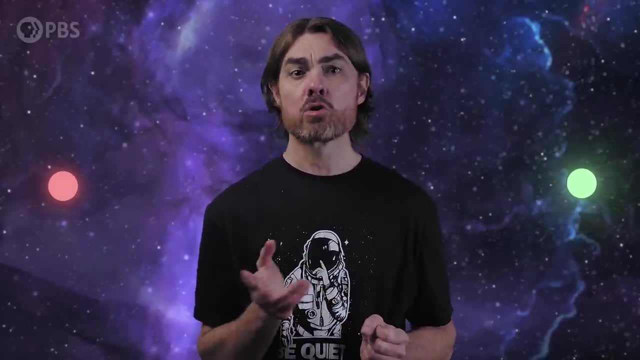 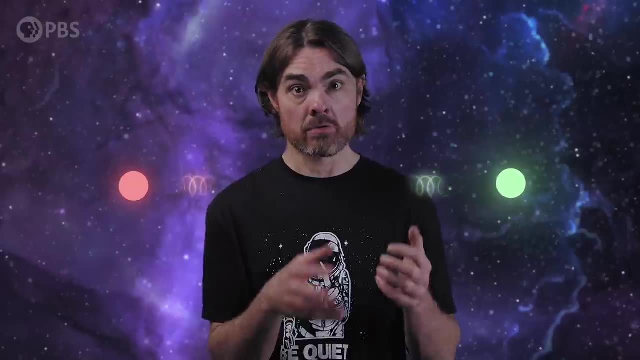 Okay, back to the strong force. Now, let's say we have two quarks hurtling towards each other. They're going to interact by the strong force, which is mediated via virtual gluons of the gluon field rather than virtual photons of the electromagnetic field. We can draw Feynman. 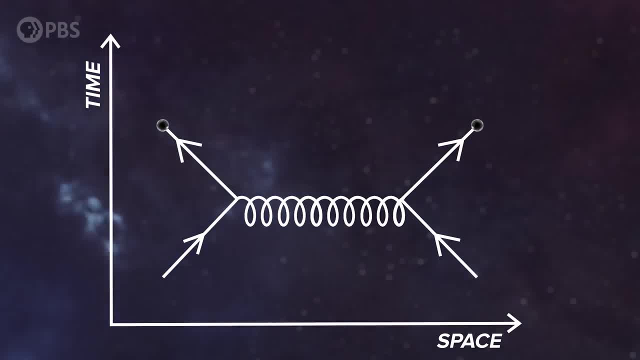 diagrams of these interactions, now with cute curly gluon lines, Presumably, then, to calculate the probability of a given interaction. we'll have to calculate the probability of a given interaction. We again just add up diagrams, with the probability of each diagram determined by the number of vertices. 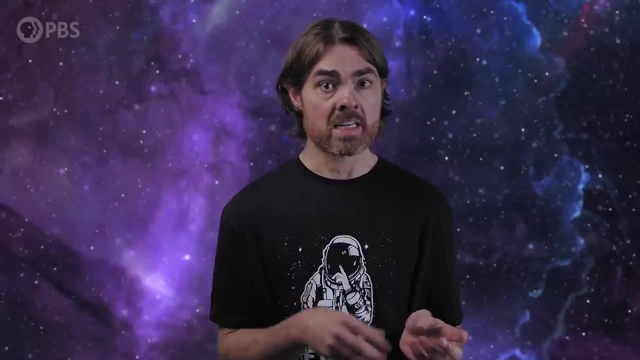 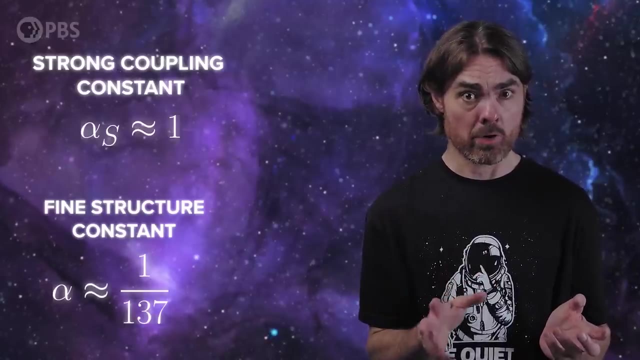 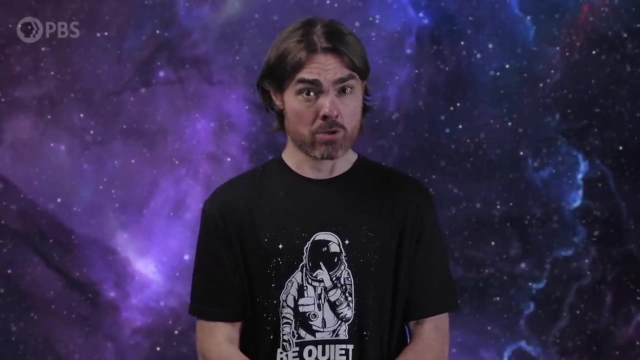 The coupling strength for the strong nuclear force is ingeniously named the strong coupling constant. It is much higher than the fine structure constant and it's of order 1, although it depends on the energy scale. That's what makes the strong force strong and it's also what makes the strong force 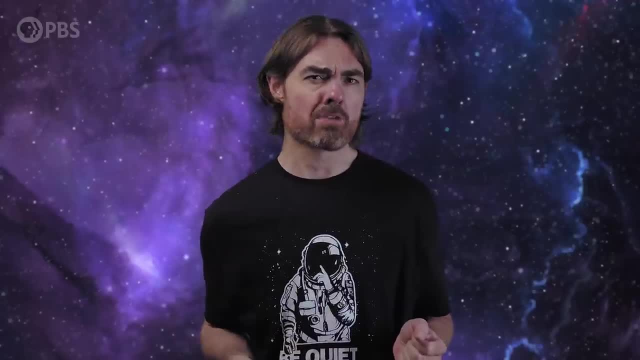 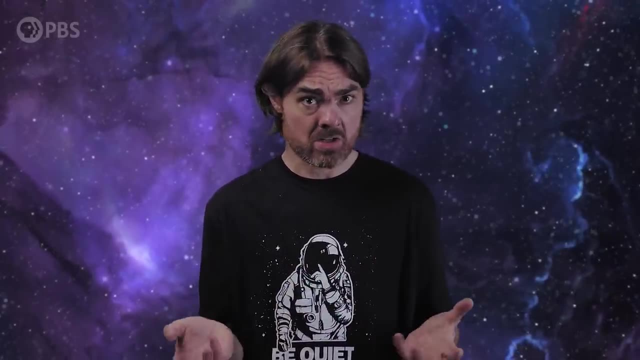 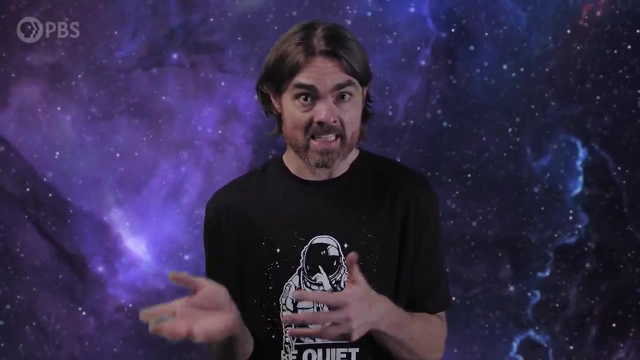 interactions very difficult to calculate. You no longer have the luxury of throwing away all but the strong coupling constant. In fact, that's when you're calculating the interaction probability for your pair of quarks. Adding new vertices doesn't decrease the probability anywhere near as quickly as with QED. This means you can't possibly do this calculation with pen and paper. 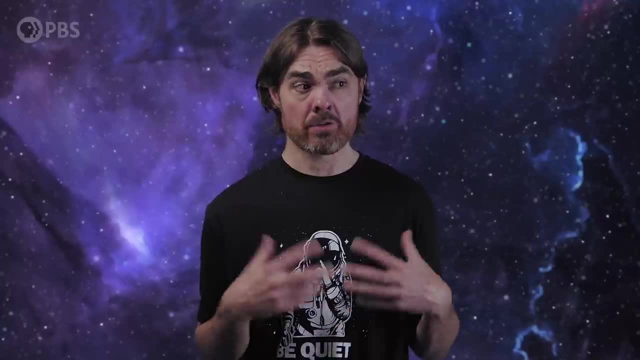 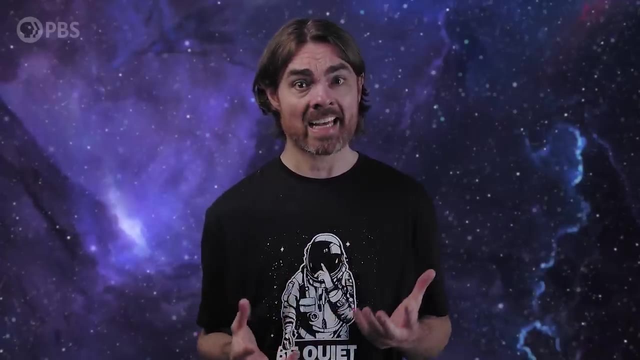 In fact, it's extremely challenging to do QCD with the Feynman diagram approach, even with computers. Now, before any particle physicists start shouting at me, I'll quickly add the caveat that there are some unusual cases where the strong coupling constant is going to be the strong coupling constant. 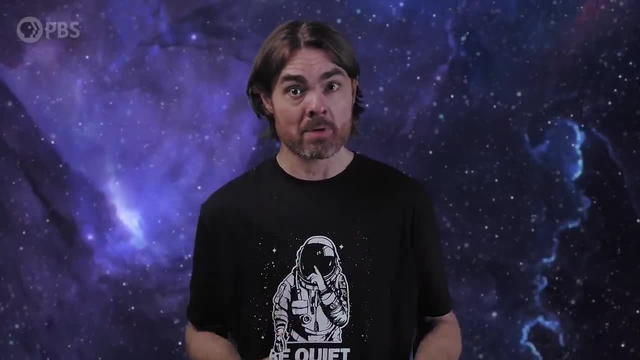 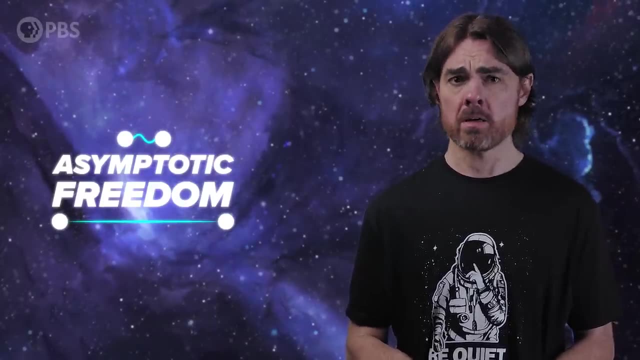 constant can become small and quarks can be understood with Feynman diagrams, and this is the phenomenon known as asymptotic freedom. but if I tried to explain that too, we would be here all day. In general, if we can't calculate what quantum chromodynamics predicts for the behavior of 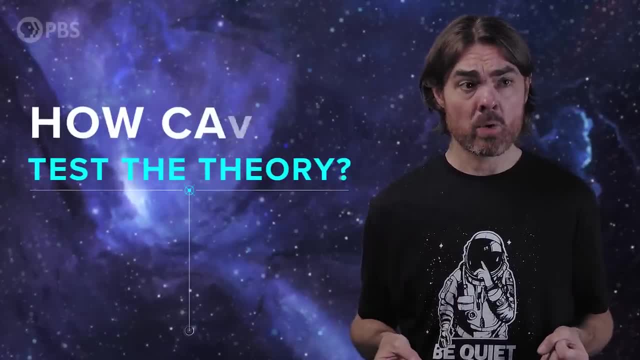 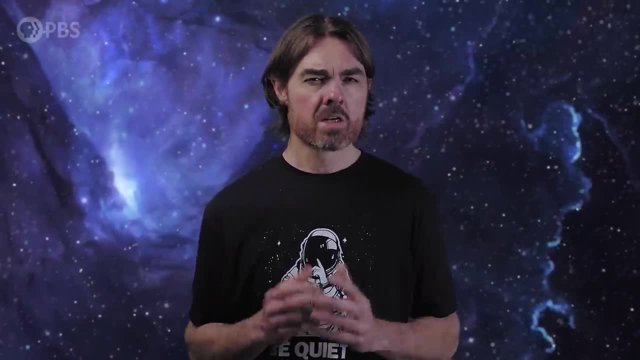 quarks. then how can we even test the theory? Well, we need to abandon Feynman diagrams. In fact, we need to abandon the idea of particles altogether. See, it turns out that the virtual particles that we were using to calculate particle interactions 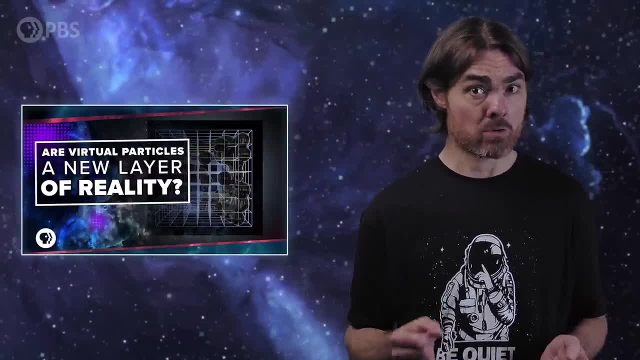 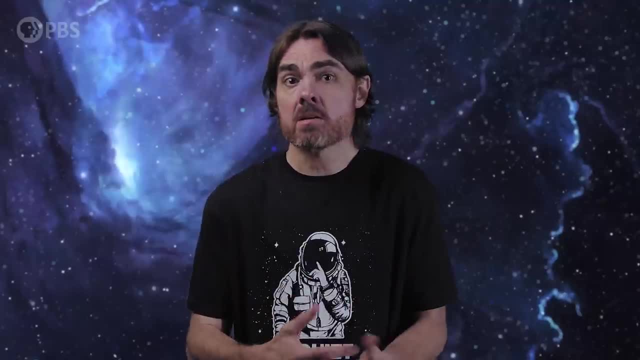 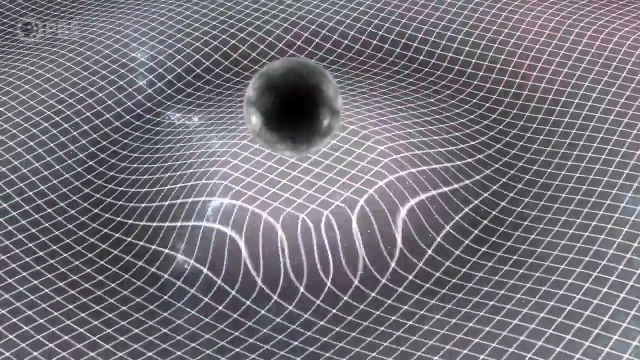 don't actually exist. We've talked about that fact recently. Real particles are sustained oscillations in a quantum field that have real energy and consistent properties. Virtual particles are just a handy calculation tool, a way of representing something deeper. They represent the transient disturbances in quantum fields due to the presence of real 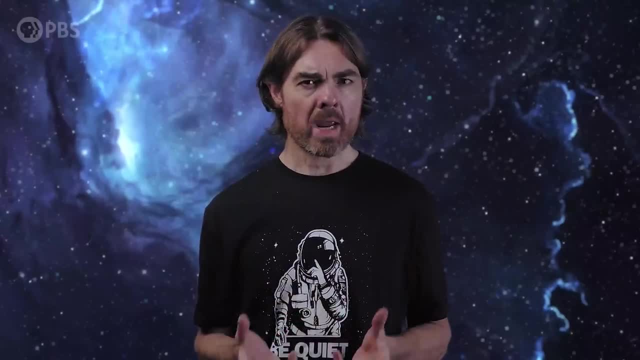 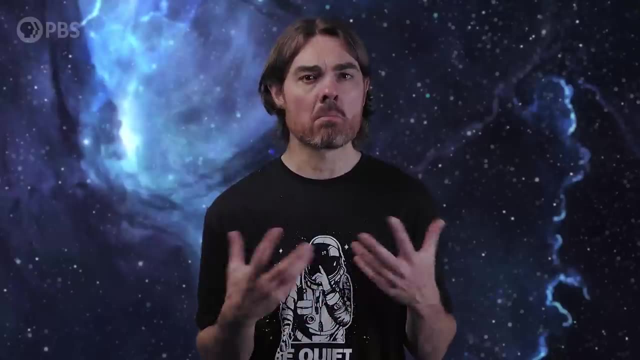 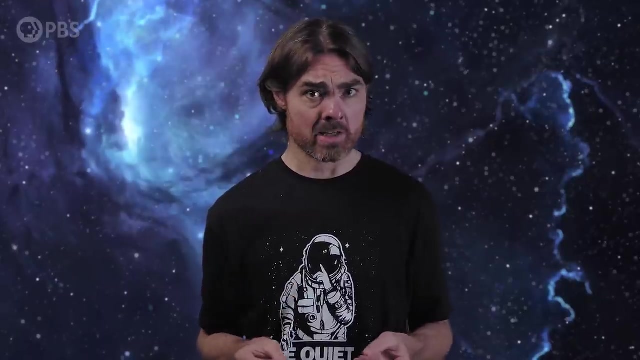 particles that couple to those fields. The coupling between quark and gluon fields is so intense that the disturbances of those fields are way too tumultuous to be easily approximated by virtual particles. Instead, we have to try to model the field more directly, and that's where Lattice QCD. 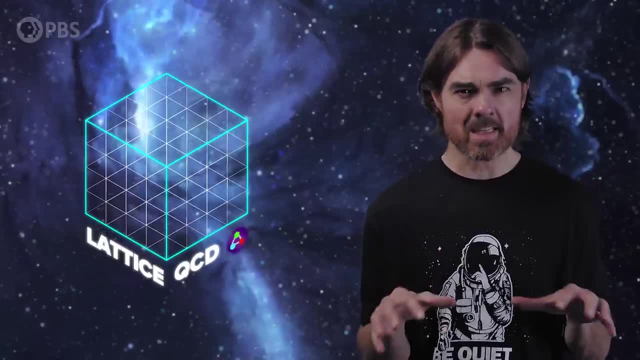 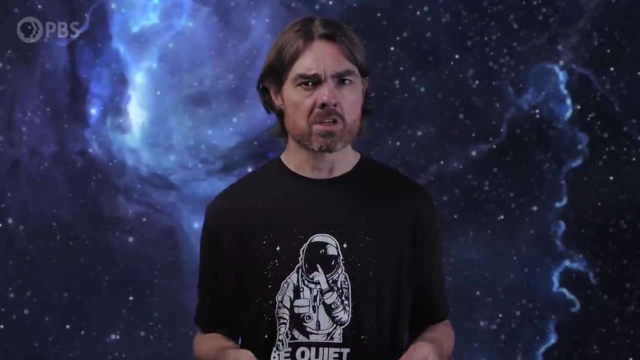 comes in. It's an effort to model how the quantum fields themselves evolve over the course of a strong force interaction, Similar to how Feynman diagrams work. to do this, you need to account for all possible paths between the starting and final field configuration to get the probability of that. 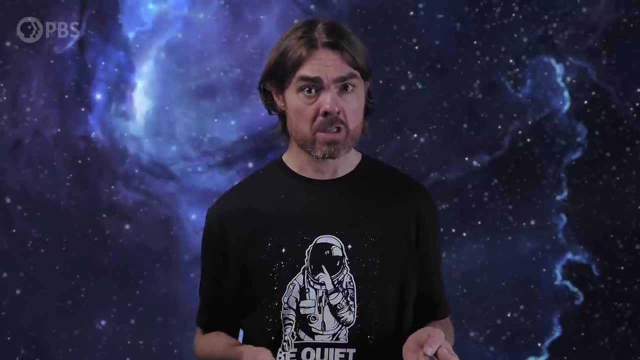 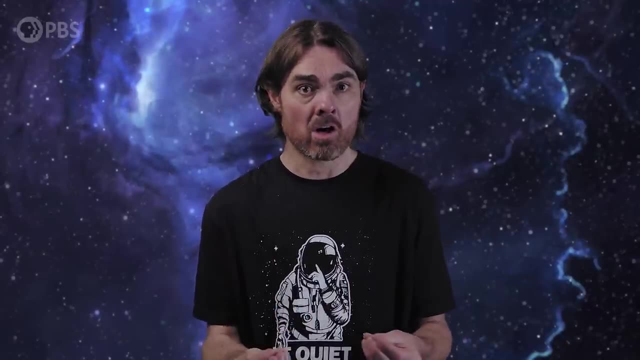 transition happening Now. there's a good reason we don't do this for electromagnetism. There's an astronomical number of configurations that the field could pass through in the intervening time. No supercomputer could do that, even given the entire life of the universe. 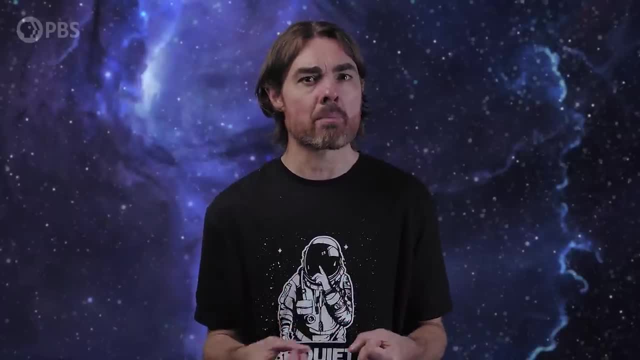 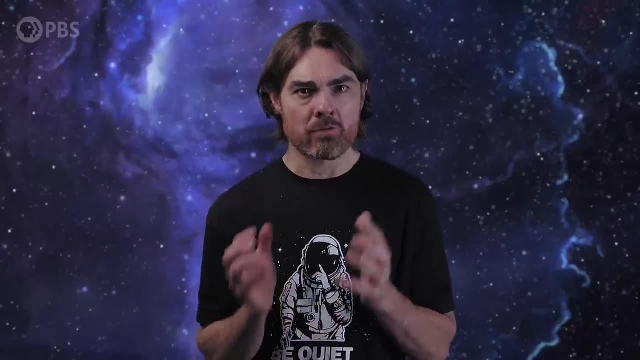 For QED Feynman diagrams, let us reduce the number of field configurations by approximating them as virtual particles. But for QCD we don't. Here we have to stick with fields, and so we need a different hack. In fact, we need a few of them. 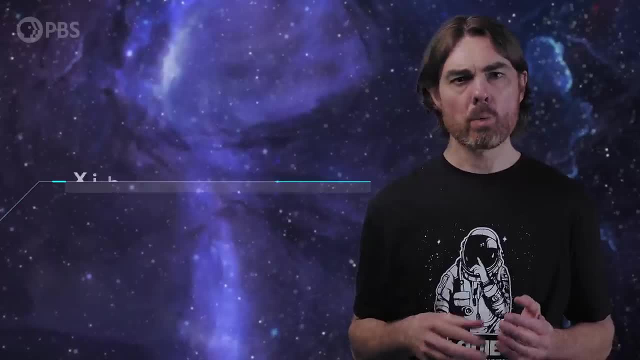 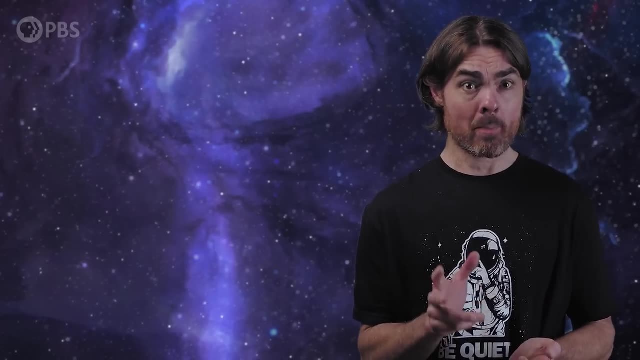 Let's make sure we understand exactly what we're trying to do here. We want the probability that some wiggly quantum field wiggles between one state and another. Let's go back to electromagnetism just for a second, because there's an analogous case. 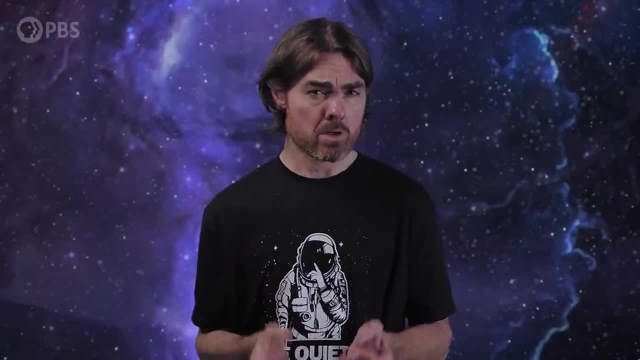 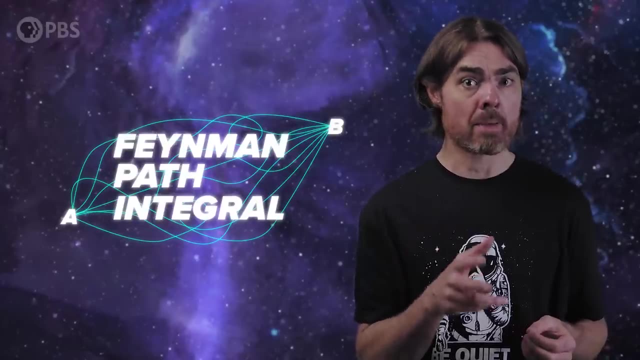 here and one that we've already covered. So before Richard Feynman came up with his famous diagrams, he devised a way to calculate quantum probabilities called the Feynman diagram, The Feynman path integral. It calculates the probability that a particle will move from one location to another by 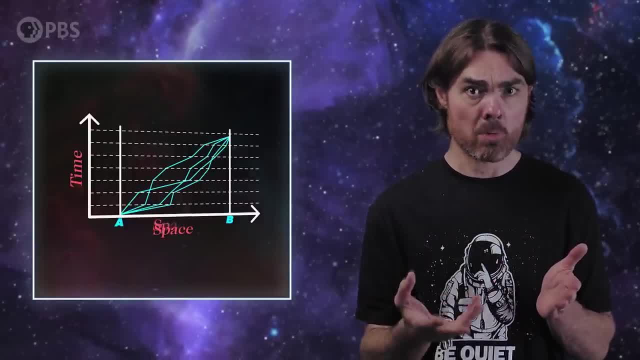 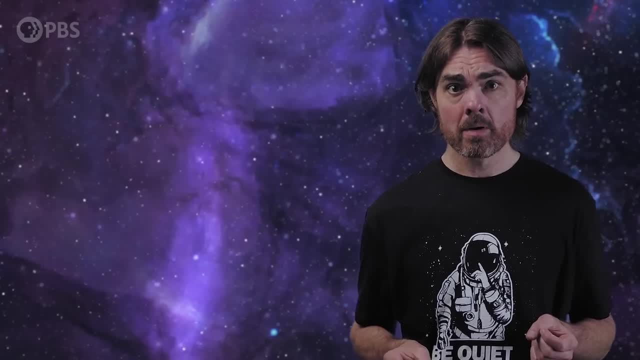 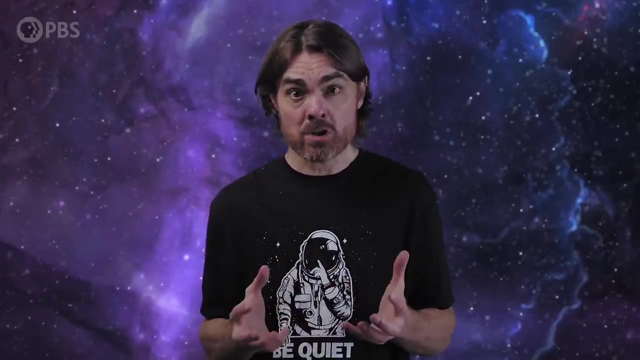 adding up the probabilities of all possible paths between those points. Actually, it also includes the impossible paths, but there's no time to explain that right now. Every time you add the probability for a single Feynman diagram, you're actually adding infinite possible trajectories using Feynman path integrals. 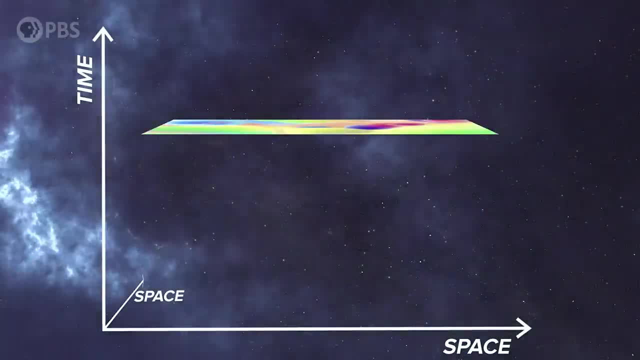 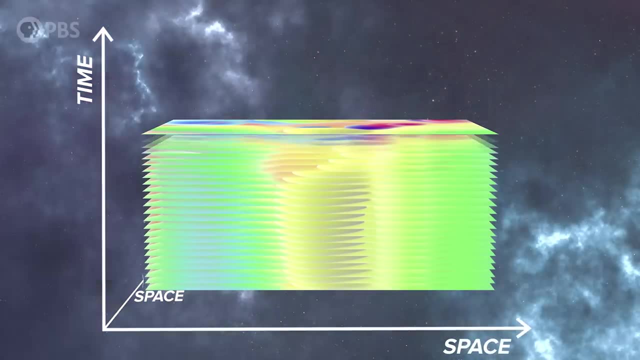 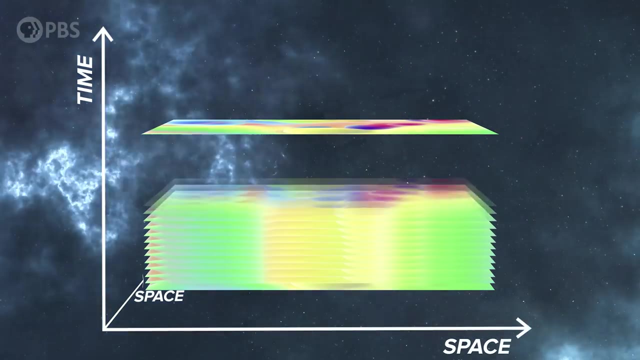 In lattice QCD We want to do something like a Feynman path integral, but instead of trajectories through physical space we add up trajectories through the space of field configurations. And that is much harder to do for three reasons. First, any patch of spacetime technically contains an infinite number of points and 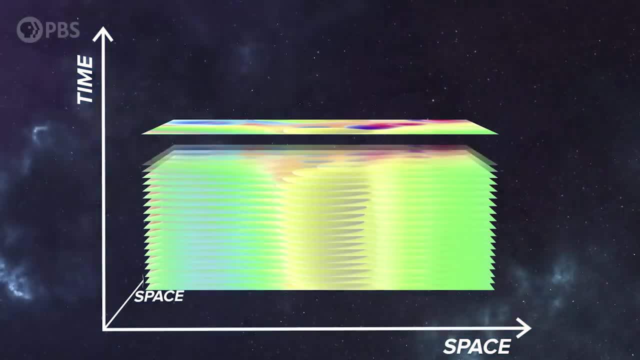 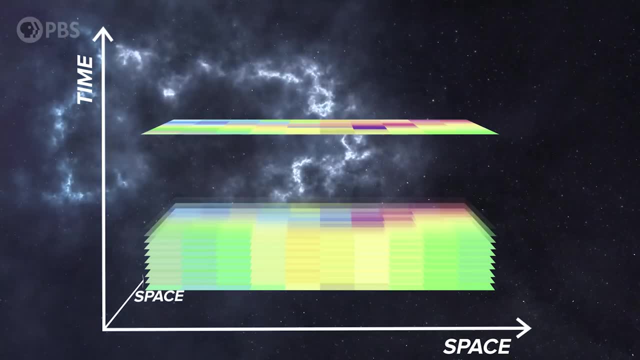 no computer can hold an infinite amount of memory. So we need to pixelate spacetime. so there's only a finite number of points. But even then there's still an astronomical number of ways that the field can move, So we need to pixelate spacetime. so there's only a finite number of points. But even then there's still an astronomical number of ways that the field can move. So we need to pixelate spacetime, so there's only a finite number of points, But even then there's still an astronomical number of ways that the field can move from. 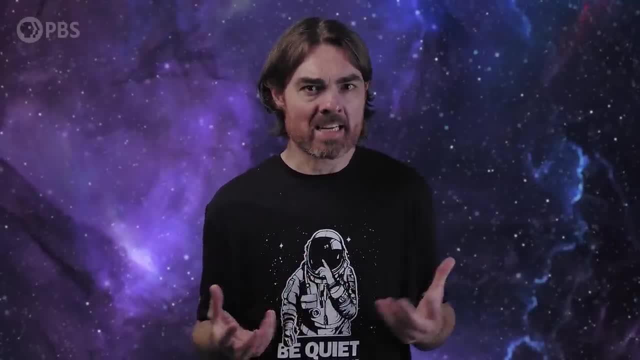 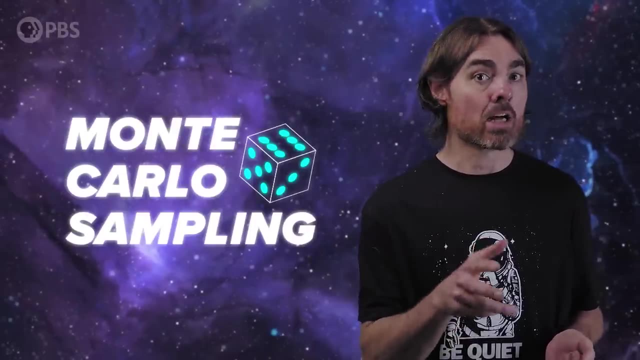 the starting to final configuration. And because these configurations are messy, we can't do a simple integration like in the Feynman path integral. So our second trick is called Monte Carlo sampling. This is an extremely common computational method in which you do your calculation based. 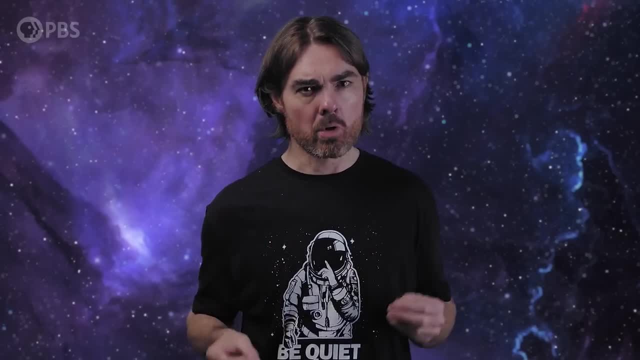 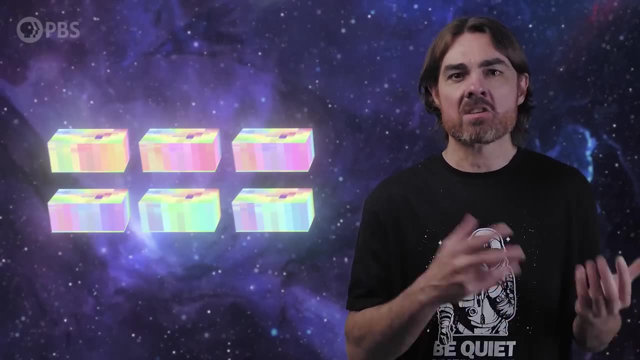 on randomized selections from some distribution. So we randomly choose a selection of field configurations of a pixelated space that get us from the start to the end of our interaction. So we randomly choose a selection of field configurations of a pixelated space that get us from the start to the end of our interaction. 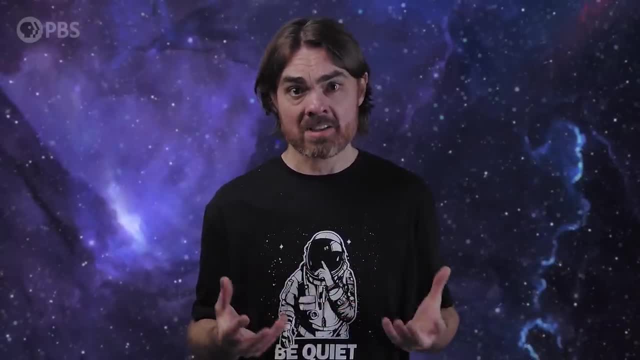 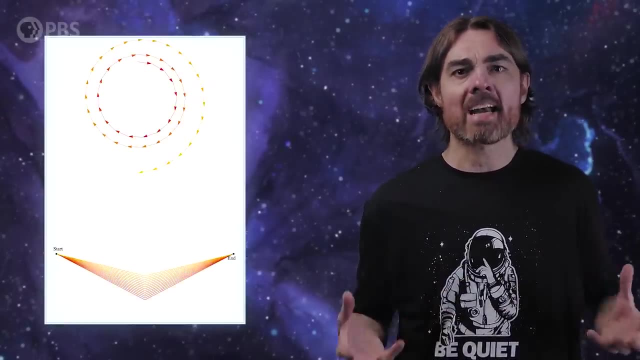 So we randomly choose a selection of field configurations of a pixelated space that get us from the start to the end of our interaction. But these can't be totally random because some of these paths are still more likely than others. In the Feynman path integral, the probability of each path comes from adding up all of the. 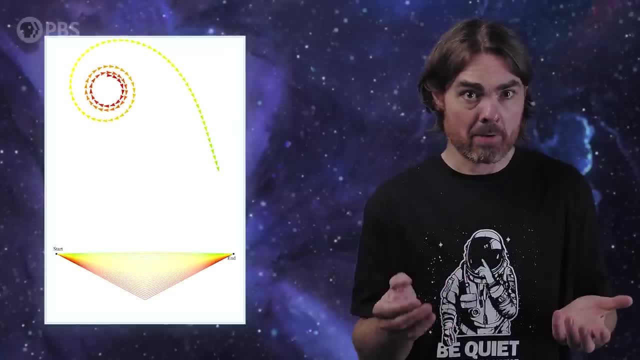 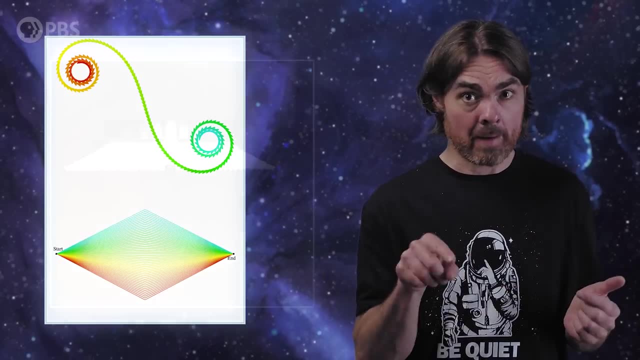 little shifts in the particle phase from each step. Then at the end of the path you add together the phases of all possible paths to get the total probability of reaching that point. This is exactly like the famous double-slit experiment, where the probability of a particle 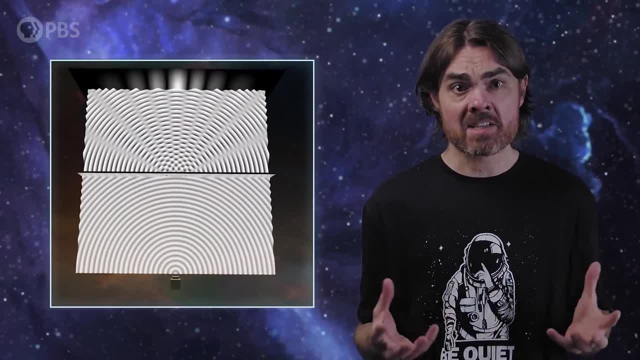 landing at a certain point on the screen depends on where the particle is. So we can't do a simple integration like in the Feynman path integral, where we add together the phases of different slits on間 and these different set of paths are a. 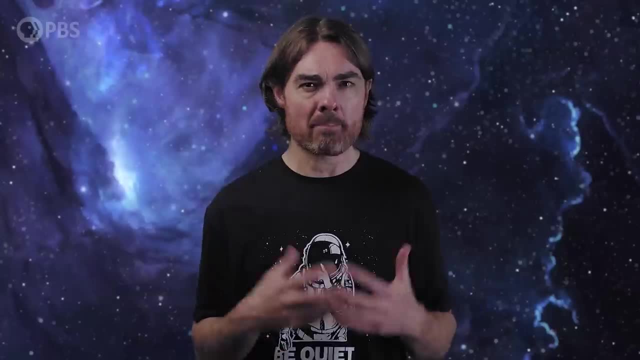 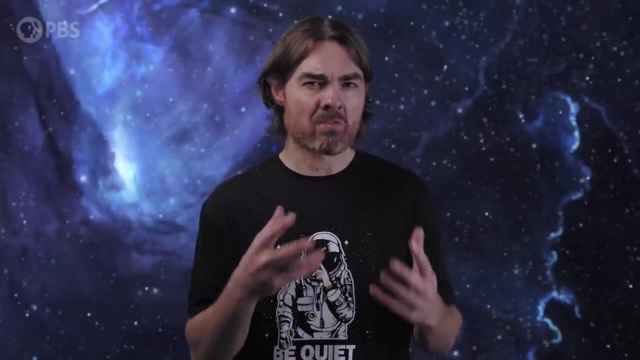 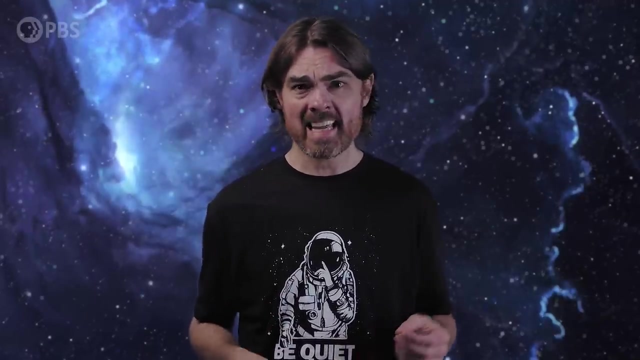 single line. Our quantum field is a 3D pixelated lattice that evolves through time. As with the Pyth integral, each timed step results in a complex-valued phase shift at each spatial point. Those complex numbers are fine in the Feynman path integral because they get squared at. 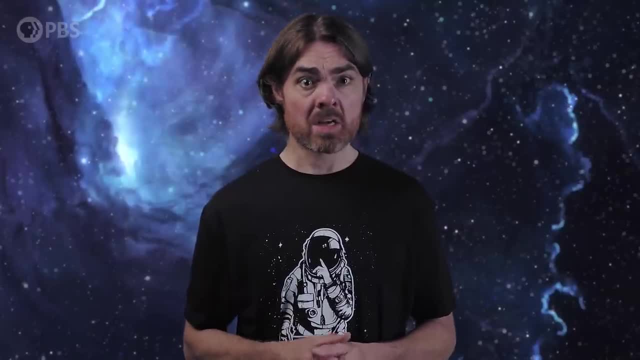 the end and disappear, but they're very difficult to deal with in the Monte Carlo approaches. So on top of that, we get this cryptвин which, however, товarming it even Hannesそして. So you need one more hack, our most ingenious yet. 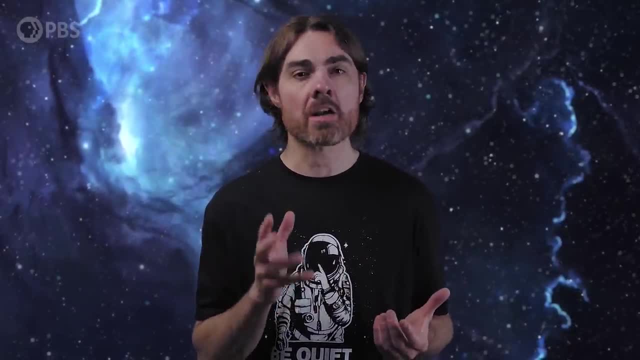 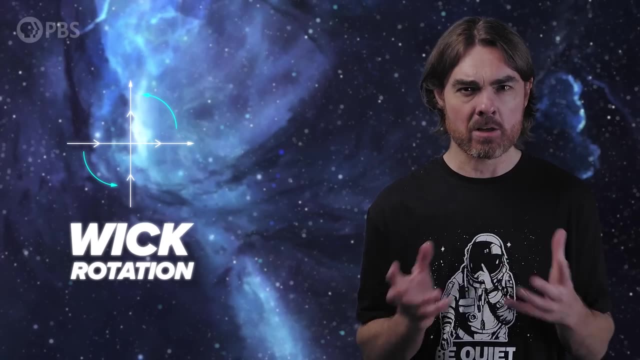 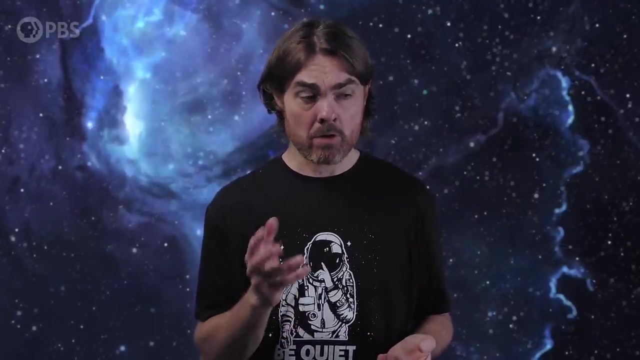 We're going to pretend that time is just another dimension of space. This operation is called the wick rotation, and it eliminates the complex nature of the phase shifts. If we then pixelate the time dimension, we have a lattice with four spatial dimensions. 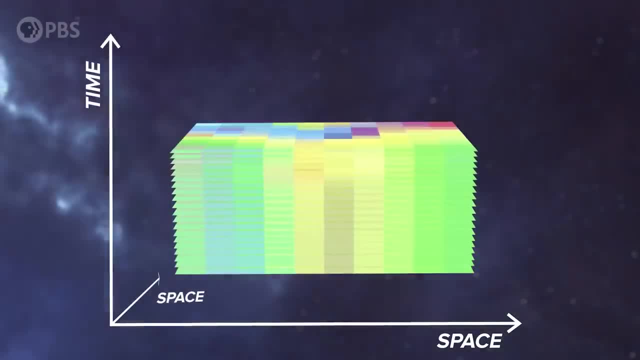 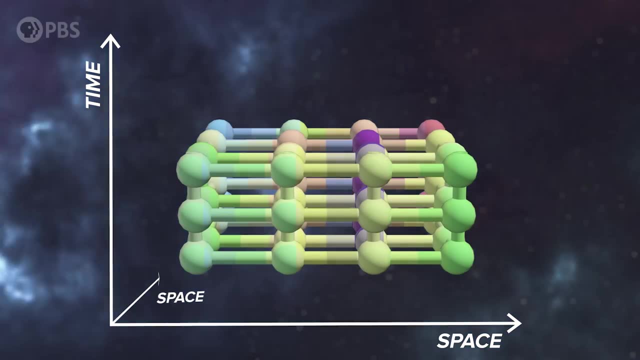 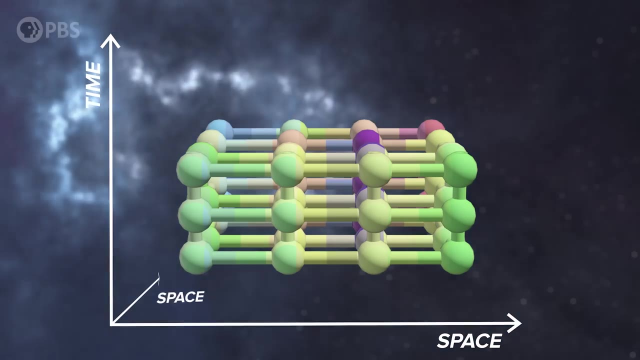 Now our coupled quark-gluon field looks like this: a lattice of points with connections. The points are the quark field and the connections are the gluon field. Getting rid of the complex quantum probabilities means that this isn't really even a quantum problem anymore. 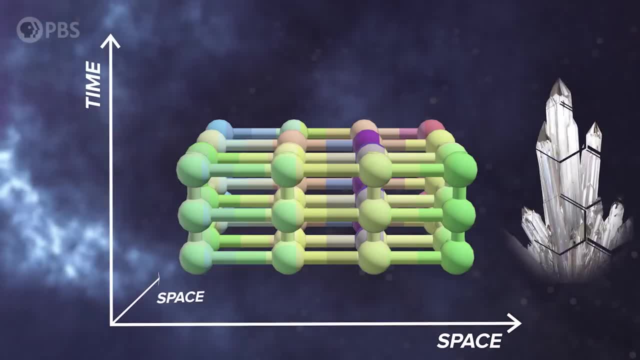 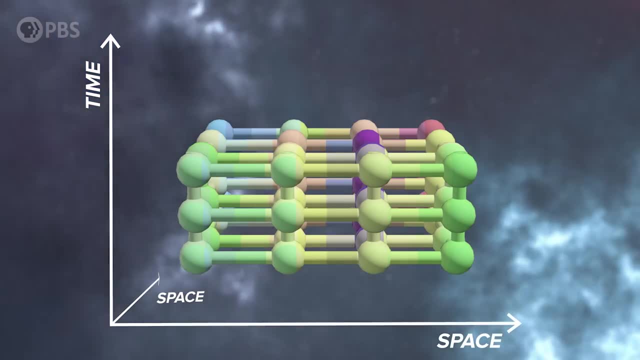 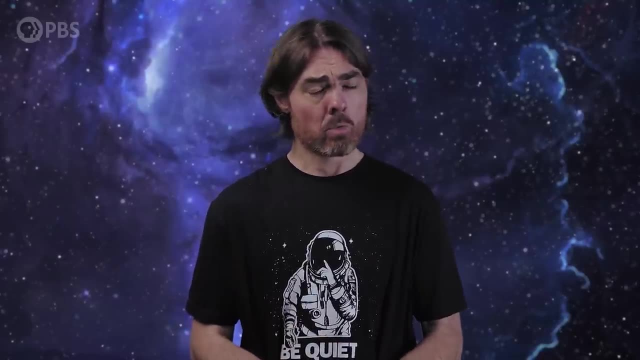 The structure just looks like a crystal, Admittedly a four-dimensional one, but a classical crystal. And guess what? We understand how crystals work extremely well. We can now simulate how this lattice evolves over time using the laws of statistical mechanics. We're not all the way there yet. After all, spacetime isn't really a discrete lattice of. 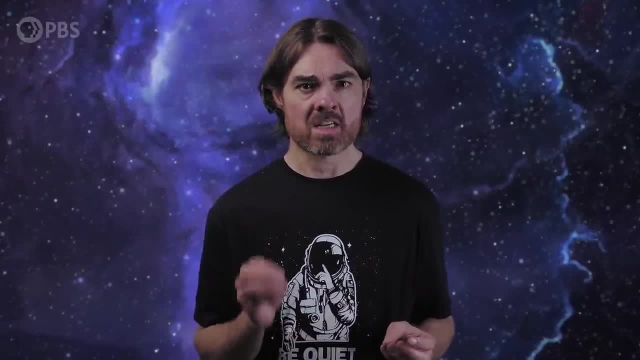 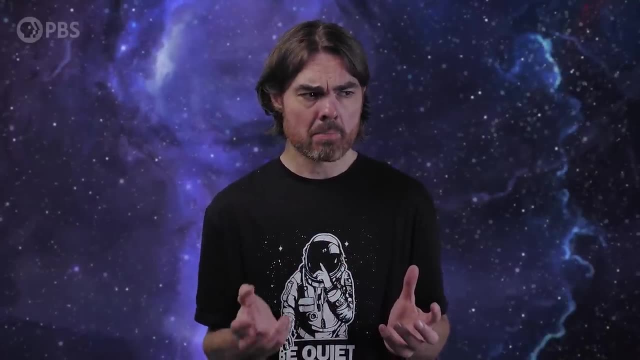 points. But it turns out that the things you want to calculate, like the mass of a hadron, actually do depend on your choice of pixel size. But they depend on it in a very simple way. You can run your simulation multiple times for different lattice spacings. 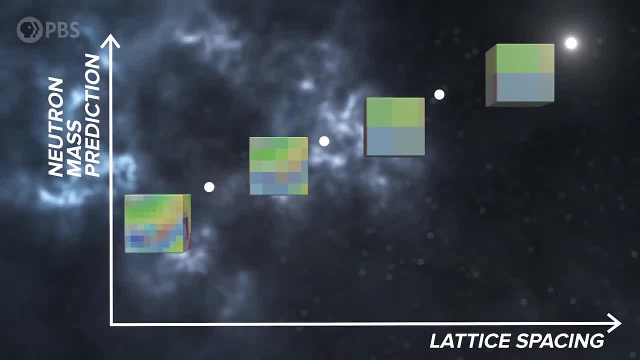 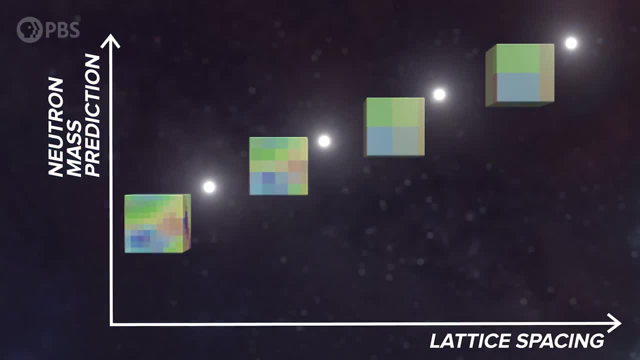 to figure out that role. It's a game of physics and you can do a lot of different things with the same method. For example, the prediction for neutron mass gets larger with increasing lattice spacing, But if you just draw a straight trend line through your simulation results. 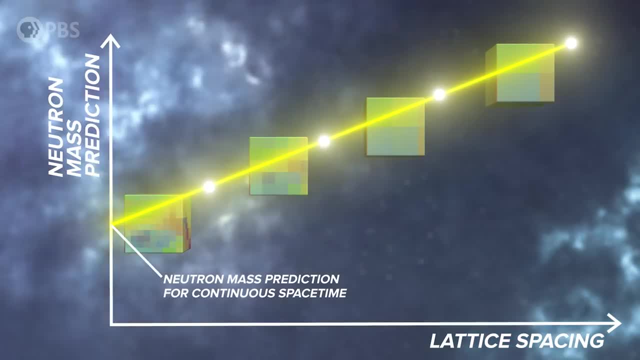 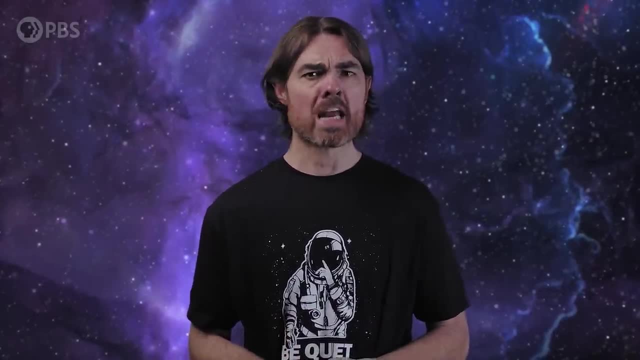 you can find out the neutron mass in the case of zero spacing, a continuous spacetime, And guess what? This gives us the correct neutron mass. This trick of transforming quantum fields into a lattice was first discovered by Ken Wilson all the way back in 1974.. Back when you'd be lucky to feel the difference, You'd be lucky to fit a kilobyte of RAM on your computer. Since then, and with the help of vastly improved computational resources, lattice QCD has accurately predicted many things from the masses and decay frequencies of hadrons. 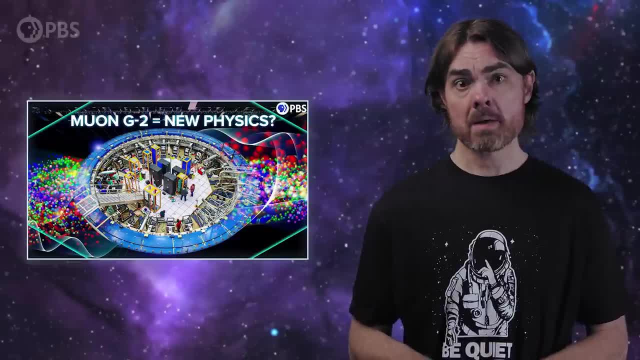 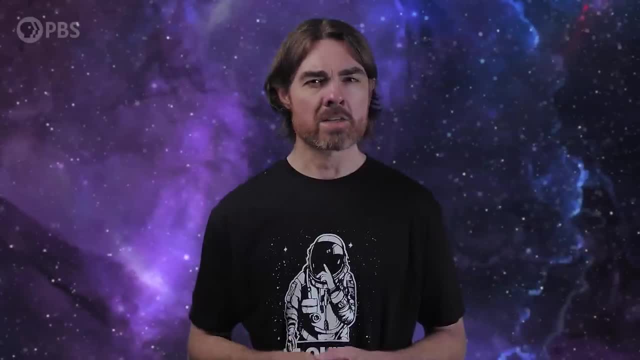 to the exotic properties of quark-gluon plasma. These simulations were also an essential part of the prediction side of the new muon G2 results. The fact that lattice QCD even works gives us deep insights into the nature of quantum fields. 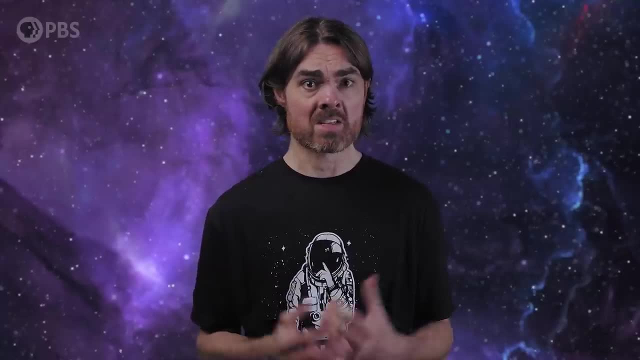 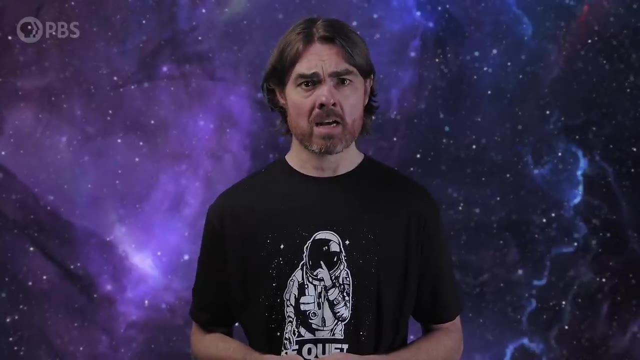 For one thing because it doesn't use virtual particles at all, but rather simulates the quantum field more directly. that helps us put to bed the idea that virtual particles are anything more than an approximation of what these messy fields are really doing during an interaction. 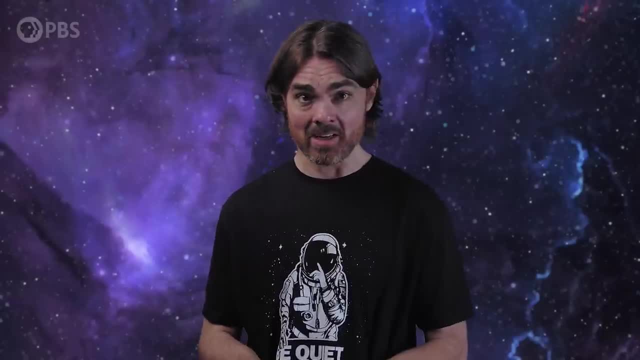 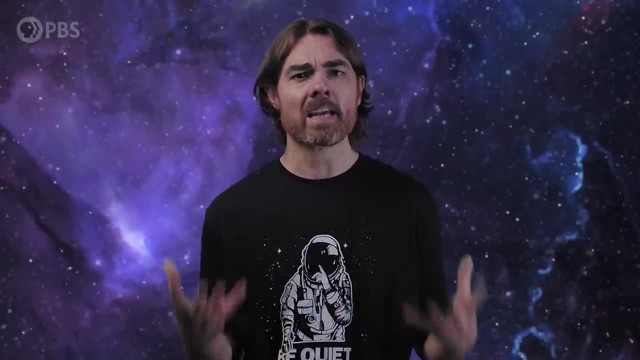 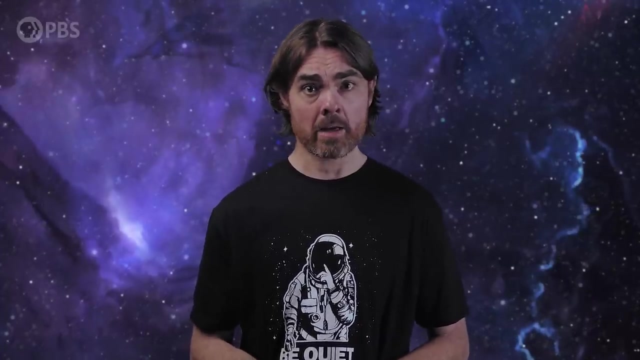 So there is your whirlwind introduction to lattice QCD. As our computing power grows, one day we'll likely be able to build detailed simulations of entire collections of hadrons, like the nucleus Of a single atom. We will never simulate a whole universe this way, nor anyway, in all likelihood. 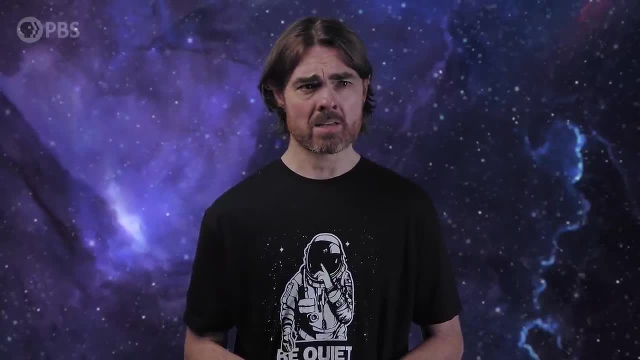 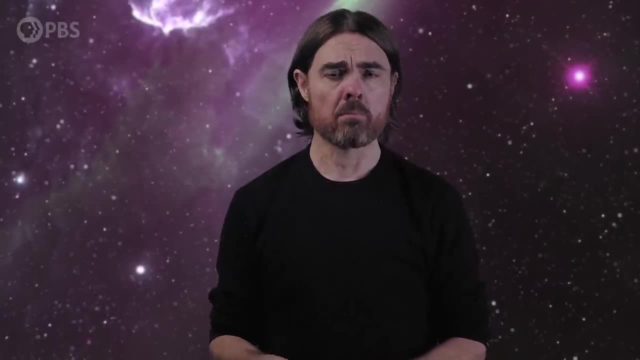 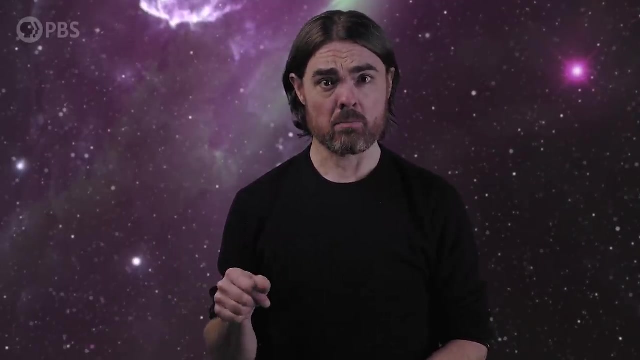 but we're going to learn so much just by simulating these tiny patches of spacetime. Before we get to comments, I just want to thank everyone who supports us on Patreon. It is incredibly helpful and greatly appreciated. If you would like to join us on Patreon, there is a link in the description. 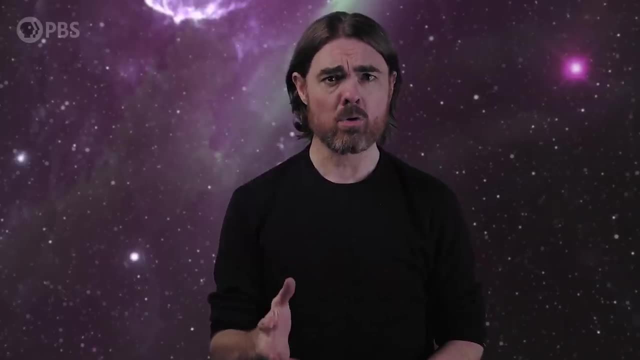 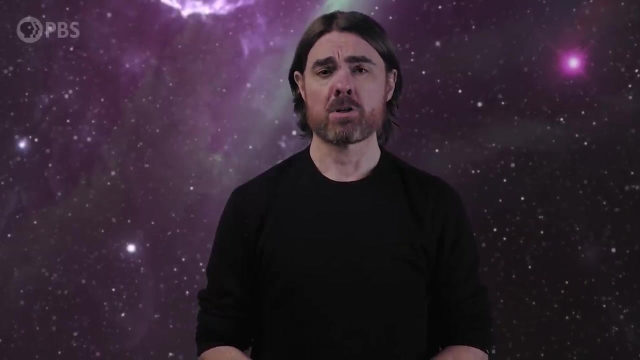 And no matter what level you join at, you'll get access to our hopping discord as well as access to every script I've ever written OK onto comments for the last two episodes. There's the one on superdeterminism and the one where we talked about what a state of matter. 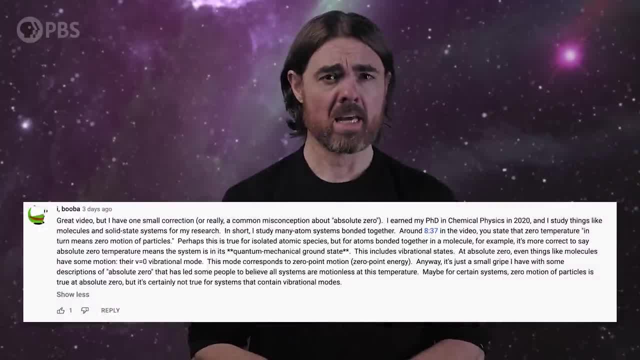 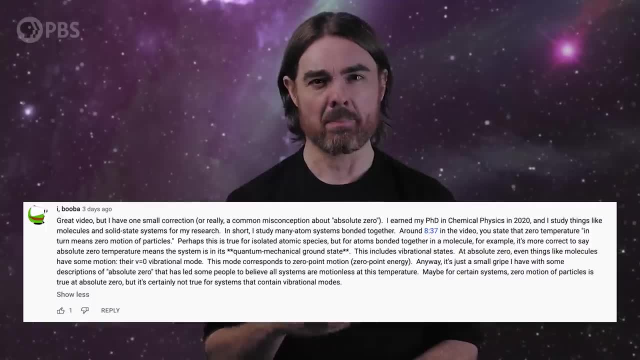 really is. iBubba points out an error in our definition of absolute zero temperature. We said that it's defined as zero kinetic energy in the particles, but actually this doesn't account for particle vibrations, which is also a place where thermal energy can lie. 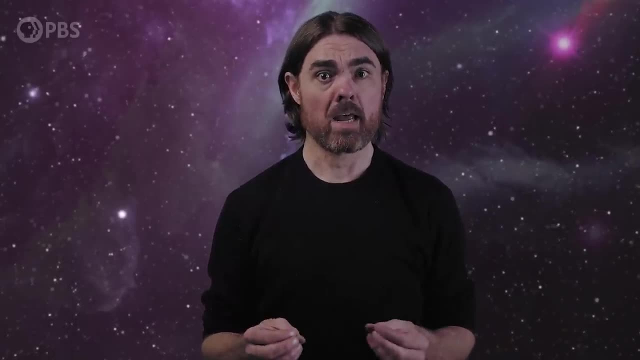 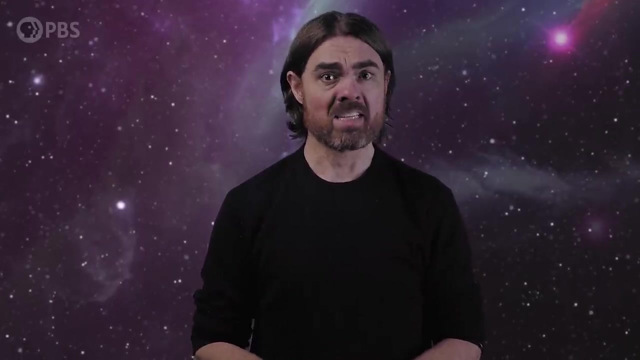 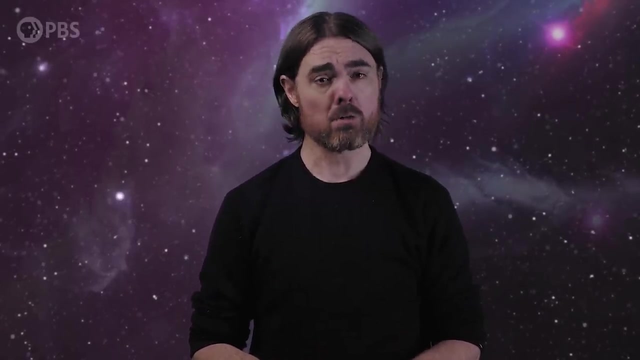 Better to define absolute zero as all particles being in their ground quantum mechanical states, And this is important because even in these ground states there's still some energy, Ground state vibrational modes, for example. So thanks for the correction, iBubba. 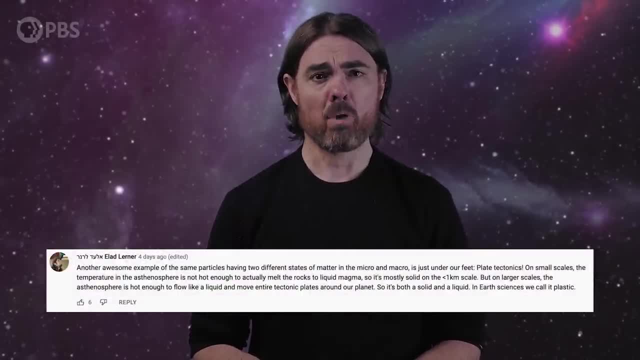 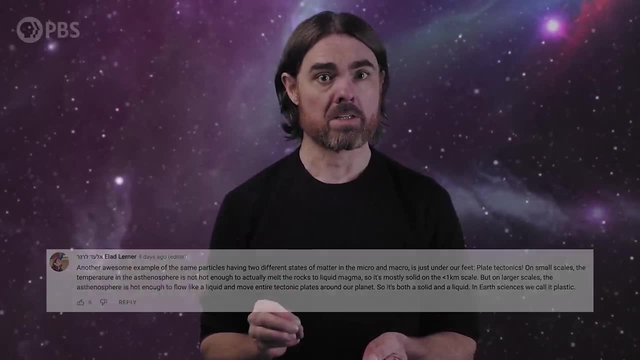 Eladlearner tells us of another example of where different states of matter can appear on different hierarchical scales, And that example is plate tectonics. Plate tectonics, The earth's upper mantle is mostly solid on scales less than around a kilometer. 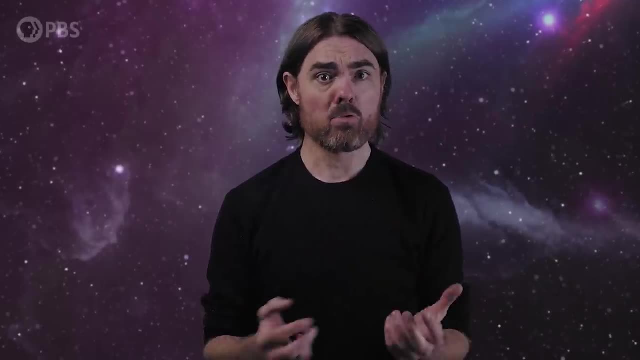 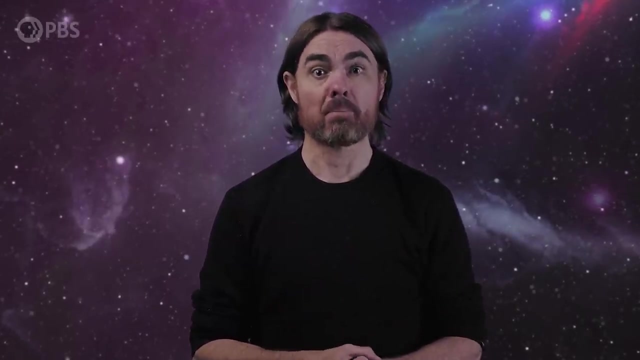 but on larger scales. it's hot enough to flow like a liquid and move around entire tectonic plates. So in a sense it's both a solid and a liquid, a state called a plastic in the earth science. Thanks for dropping the wisdom, Elad. 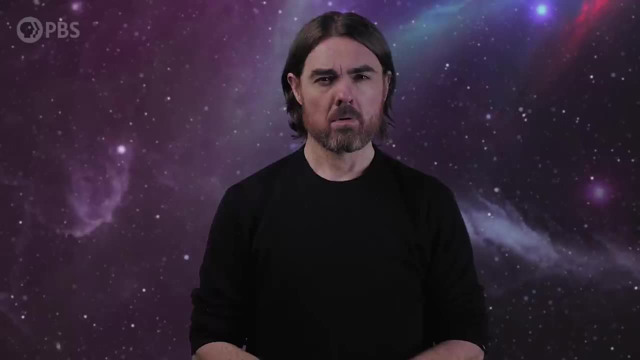 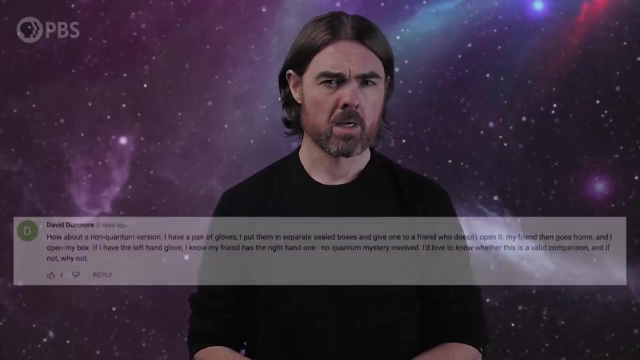 OK, moving on to superdeterminism, I would compliment you for asking so many excellent questions, but I guess you really didn't have a choice in the matter. David Dunmore proposes a non-quantum version of the EPR paradox experiment. 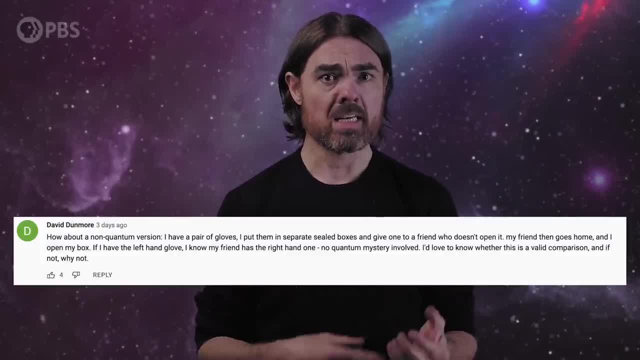 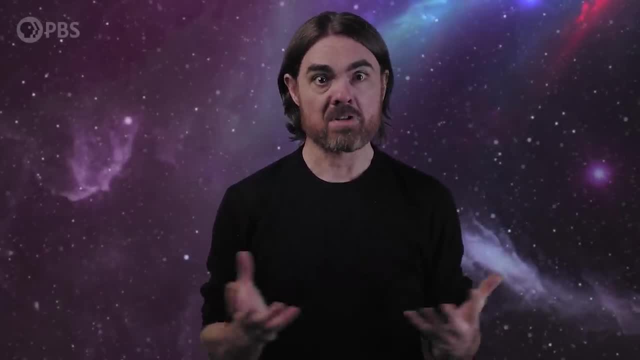 Take a pair of gloves, put them in separate sealed boxes and give one to a friend randomly. When you look in your box to see that it's the left glove, say, then you instantly know that your friend has the right glove. 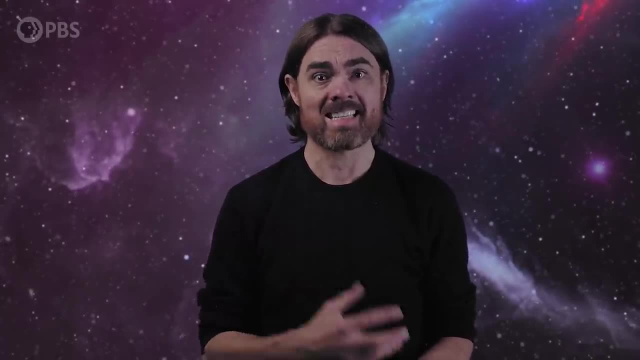 David asks whether this is a valid comparison to the entanglement experiment done with a pair of electrons with undefined but opposite spins to each other. In the case of the electrons, they're not the same. The experiment is not the same. The experiment is not the same. 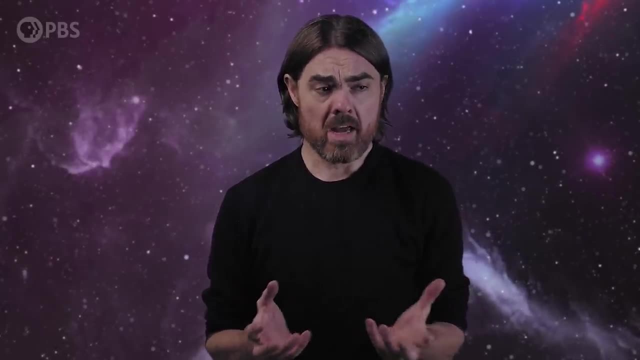 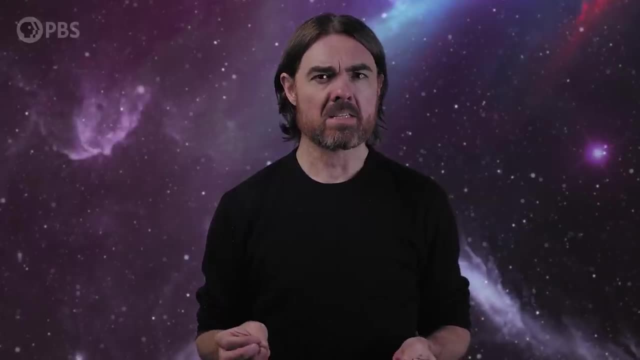 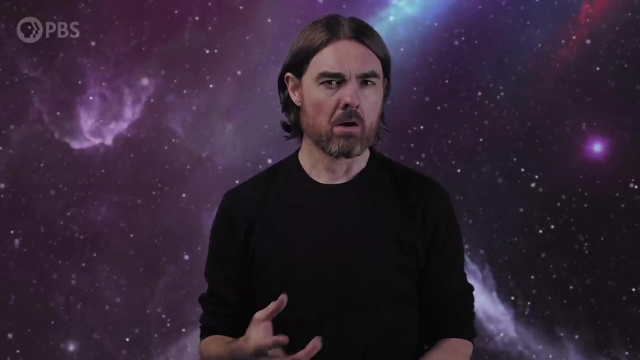 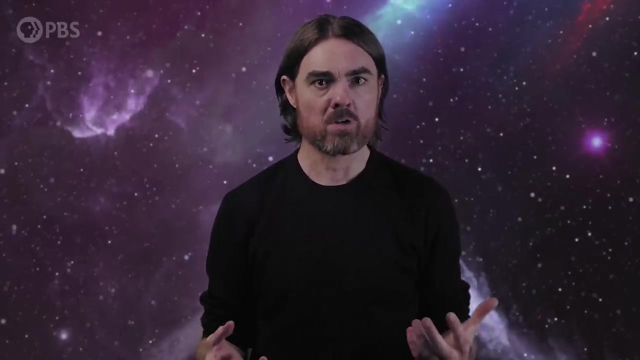 both up and down at that same time, And that means the actual direction of the spin gets randomly chosen at the moment of measurement. Now, if the spin direction is only up or down, it might be impossible to tell the difference, whether randomization happens when you put the electrons or gloves in the box or when 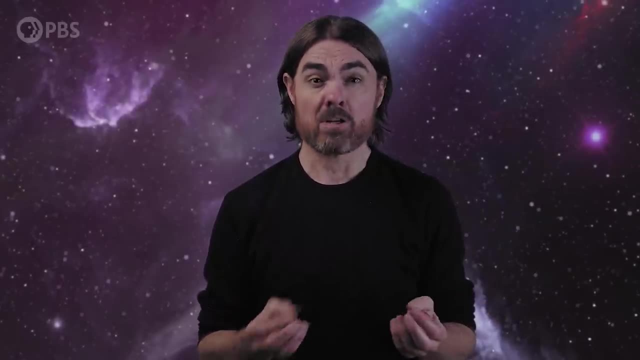 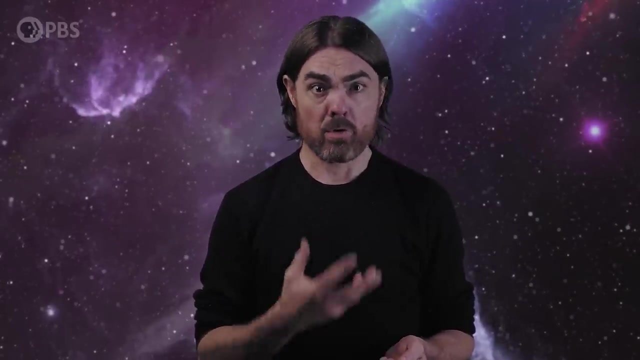 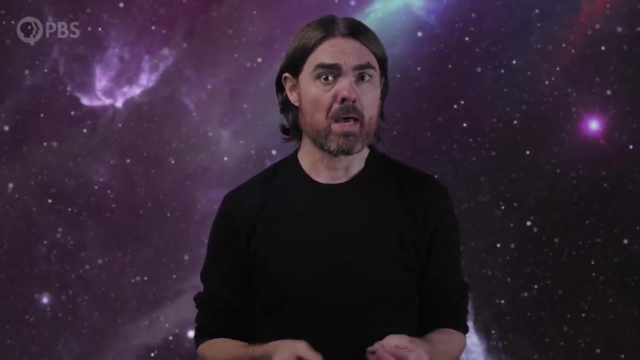 you open, the box works. But electron spin also has a directional axis- either up-down, left-right, forward-back- and that gets defined by the choice of your experimental axis. at the moment of measurement You'll always measure a fully up or a fully down electron, no matter what direction the 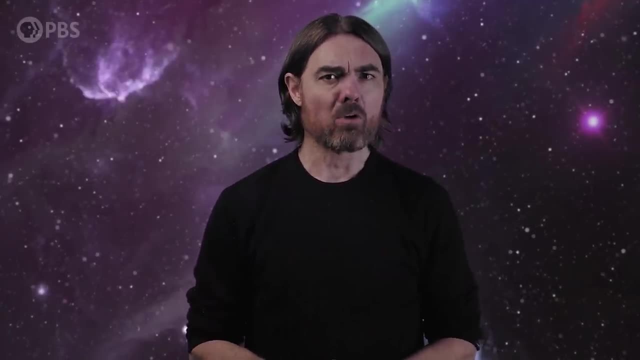 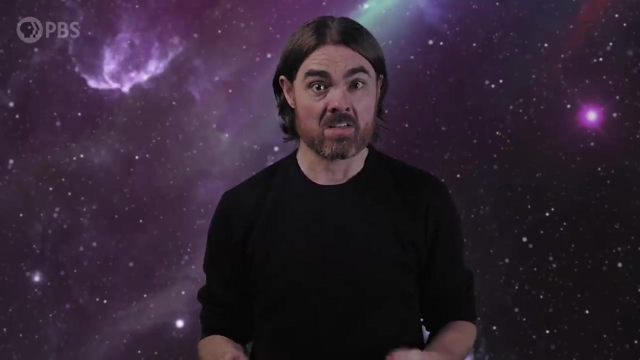 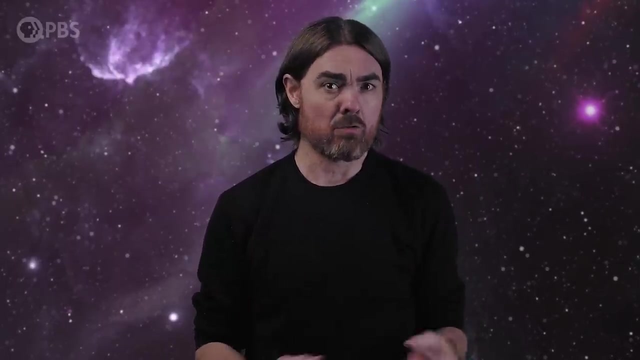 spin was initially prepared in. Its entangled partner then has to have opposite spin, but that opposite spin is going to be along the same axis that its partner was measured in, And it's the correlation between the spins measured for one electron and the choice of 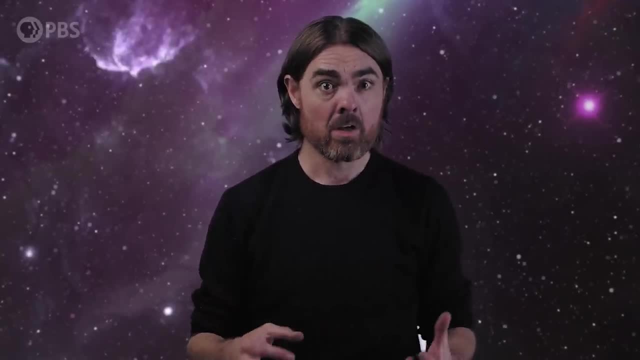 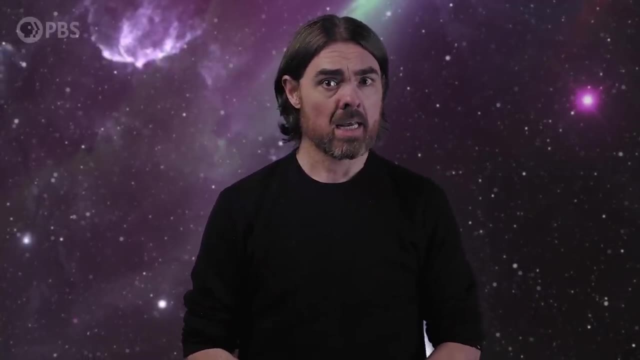 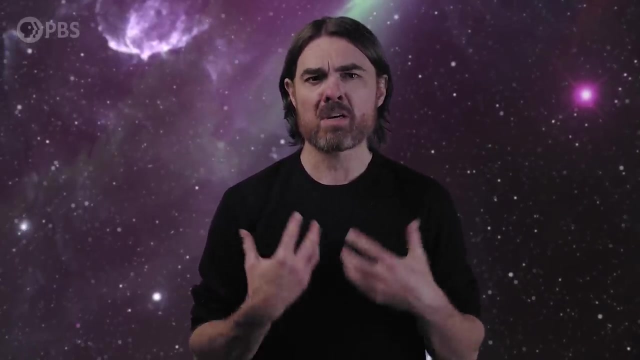 the direction of the measurement axis for its entangled partner. that is the subject of the Bell test and the source of all this spookiness. And yes, it seems that the spin direction really is set at the instant of measurement, unless, of course, our choices of measurement direction. 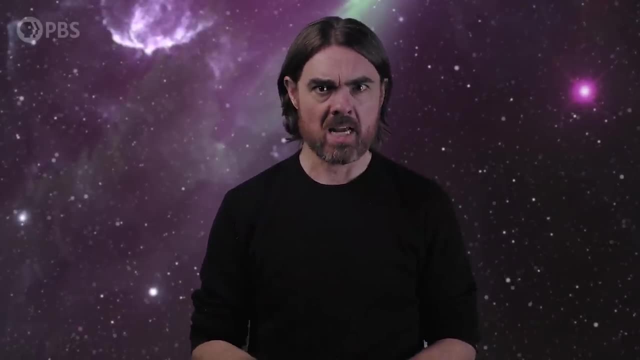 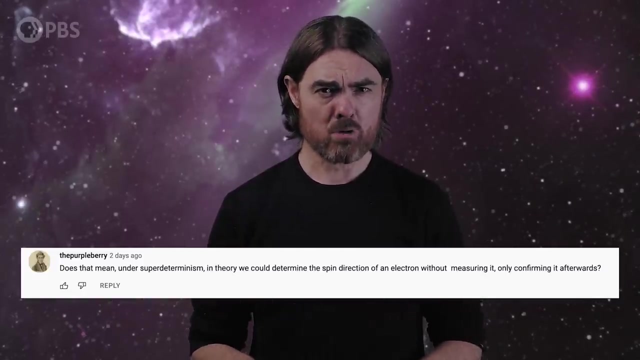 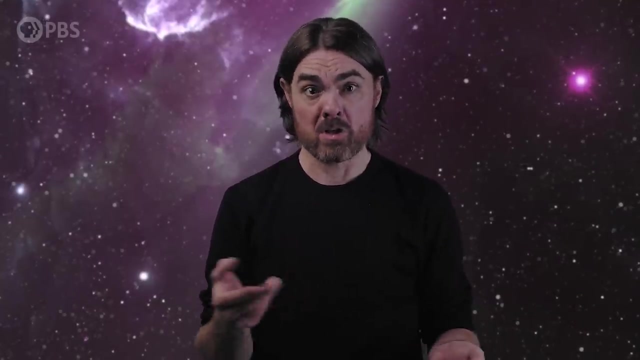 are enforced, which is what superdeterminism is saying. The Purple Berry asks whether, under superdeterminism, we could determine the spin direction of an electron without measuring it, only confirming it afterwards. Well, actually, entanglement lets us do that without even resorting to superdeterminism. Like the glove-in-the-box analogy. if you can measure the spin of an electron's entangled partner, then you know what its spin is. However, that measurement isn't a passive measure. It's a passive act. You will have actually forced the electron spin to be in some direction. based on that.